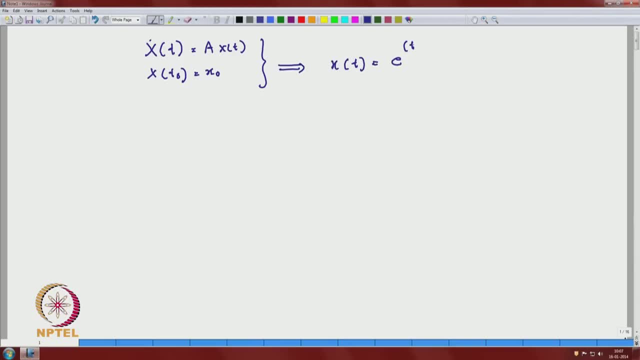 have. this is a unique solution given by e power, t minus t naught, a x naught. As I said, it has disadvantages. One is the thing: computation of an exponential of the matrix is generally difficult and secondly, it does not reveal anything about the solution trajectories. 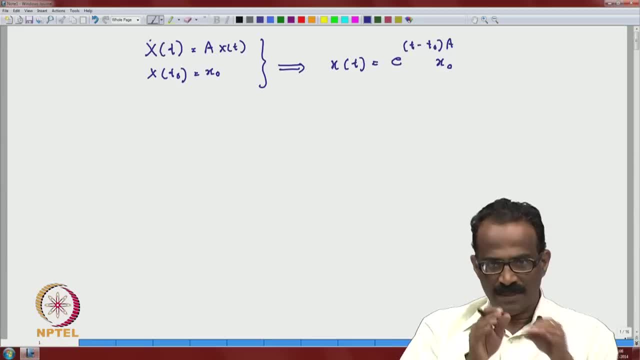 So today, this is a scenario. In this scenario we have introduced what is called the linear equivalence, whether the matrix A can be linearly equivalent to another matrix, and this is nothing but the similarity of the transformations. So when you have A is similar to B via an. 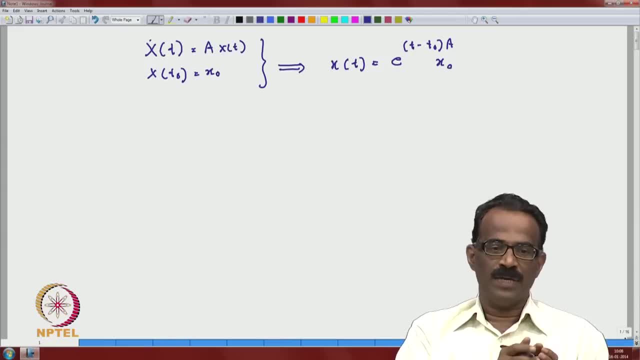 invertible matrix B. the system corresponding to A, as I called as the system 1, which is B, can be converted to a system corresponding to B, something like y, dot equal to B, y, t. And if the system B is corresponding to the system corresponding to B is c, c, 2, the exponential 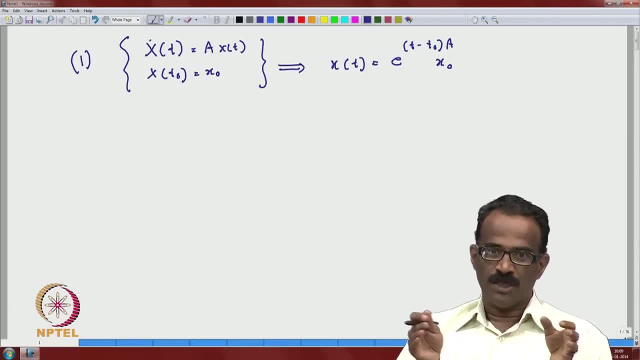 is c, c 2 compute, then the solutions will change and this change is only a coordinate change And the nature of the equilibrium point which we have introduced yesterday will not change. if the equilibrium point is stable, it will be stable for even for. 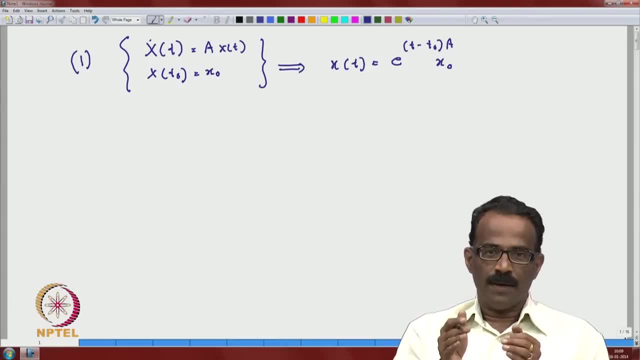 the transformer equation. So what we are. we will be going to see a detail analysis of two by two systems, which is much more simpler. In particular, if you can get the matrix B to be diagonal, saying immediately solution can be written. and 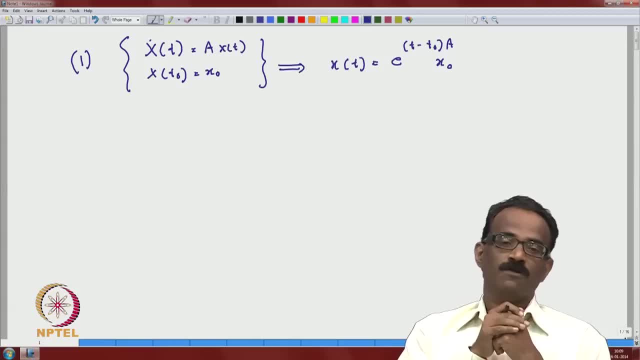 this is called the diagonalization of the matrix. But, as we know from the linear algebra, not that every matrix can be diagonalized, and that is what we have seen. a particular matrix- lambda- 1, 0 lambda- cannot be diagonalized. That is a simple, one example. because the diagonalization 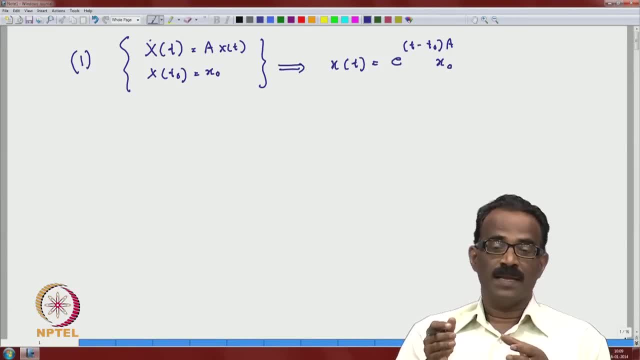 is something like equivalent to the existence of n independent eigenvectors which may not be available to you. What best we can do is what is called the Jordan decomposition, but this Jordan decomposition in 2 by 2 systems is much more easy and we will have a complete. 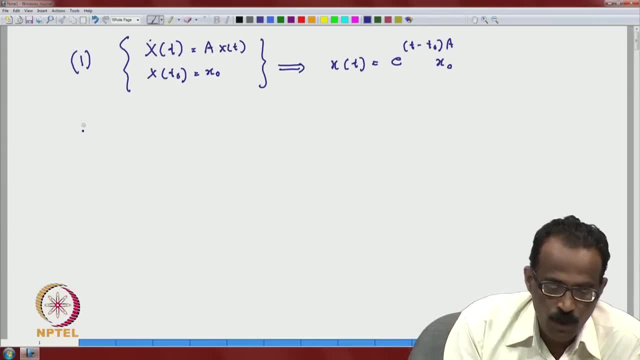 analysis today. So in this scenario, we are going to introduce what is called a phase plane, We introduce the phase portrait, We will do all this in the form of examples and we will introduce after that what is called a dynamical system. 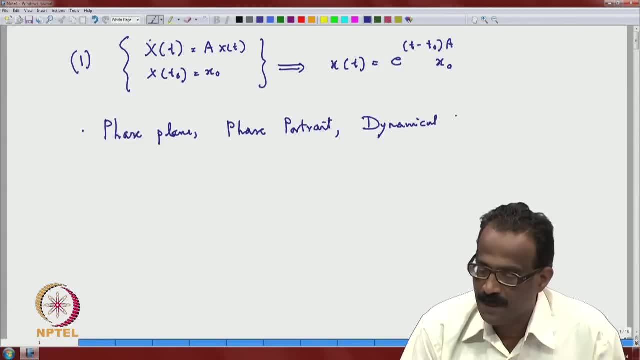 corresponding to this: 1 dynamical system. These notions we will see through example 1 and 2.. and the system we will also the concept of flow and vector field. You see all these notions quickly, I will recall, but you will also see these notions in more detail when we study. 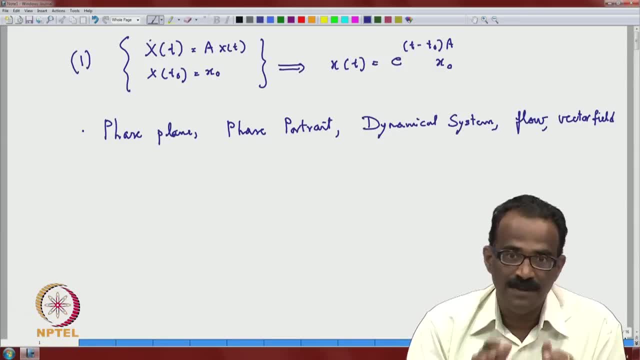 the non-linear system. So, as I said yesterday, this module is a precursor to the non-linear system and that is what: more interesting problems you will see, more interesting applications, we will be able to see these things. So let me start with the example. that is why the best way to easy. So let us look. 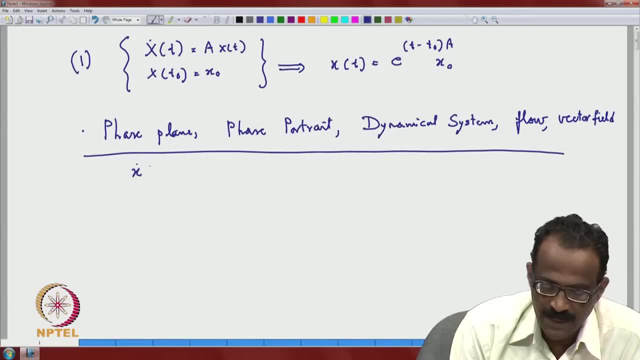 at a very simple example, x dot of t is equal to a of x t. with x at, say, you can put at any point, in particular, you can put at 0, because of the autonomy, autonomous system. What is a? I am taking to be a very diagonal matrix of the form 1, 0, 0 minus 2.. So this is a decoupled 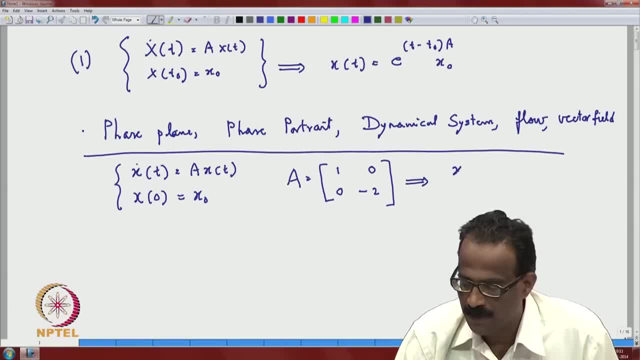 system. So the this system is nothing, but you have: x 1 dot t is equal to x 1 t and x 2 dot t is equal to x 2 dot t is equal to minus 2 x 2.. Now you know how to write a. 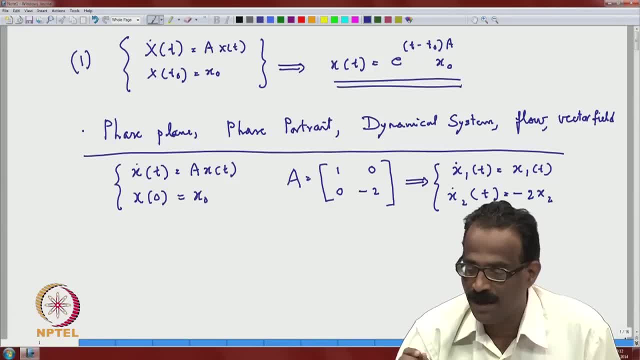 formula with the solutions like: either you can directly use this formula because it is a diagonal matrix, So you know how to compute that, or you can solve here. whatever it is, the solution will look like this: the solution of x- t is nothing, but it is at the 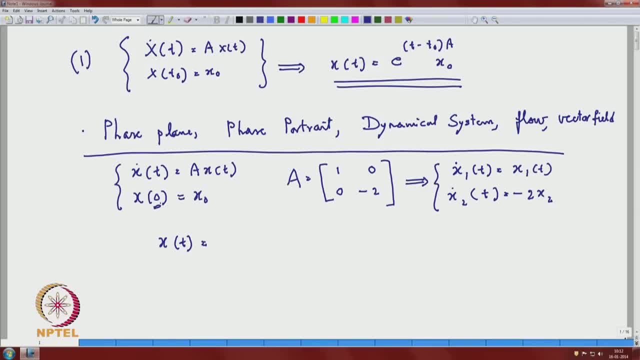 origin say it is 0, we are trying to do it and hence the solution written as e power a t. e power a t is nothing but e power t 0, 0. e power minus 2, double 1 0 minus 2.. So 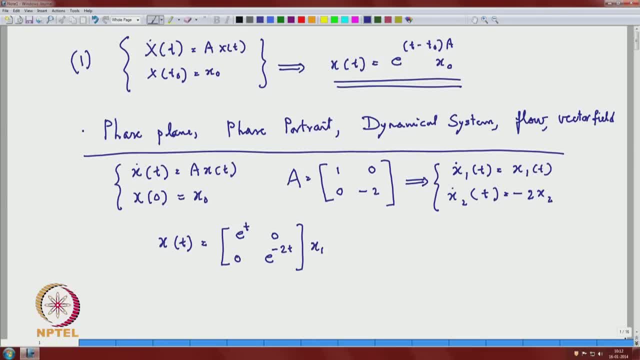 minus 2, t, x, naught. If you want it in the component wise, you will have x 1, t. So what? if you want to learn this course, You have to work this kind of more and more examples here. So you will have the solutions: e, power, t, x, naught, 1.. What is the first component? 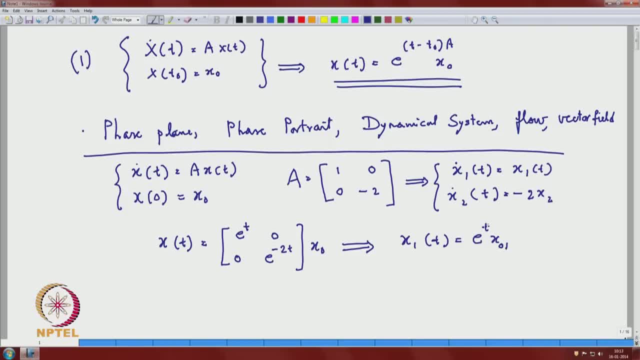 of x naught. x naught has two components, So this is x naught 1, and x 2 t is equal to e power minus 2 t into x naught 2 t. Now here is where I want to tell you something. 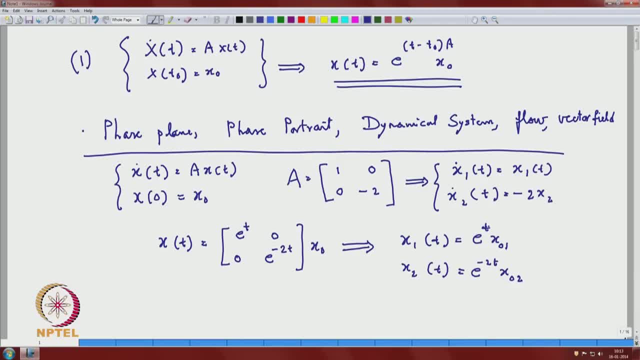 As I said, t is a time which is treated as a parameter, but this motion of x 1 t, x 2 t, the curve x 1 t x 2 t, if you write it, this is equal to your x or t. This moves in. 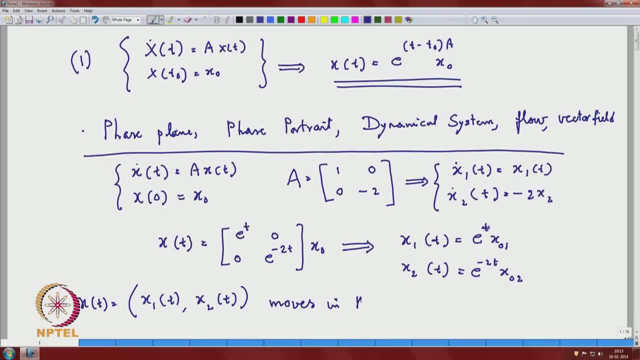 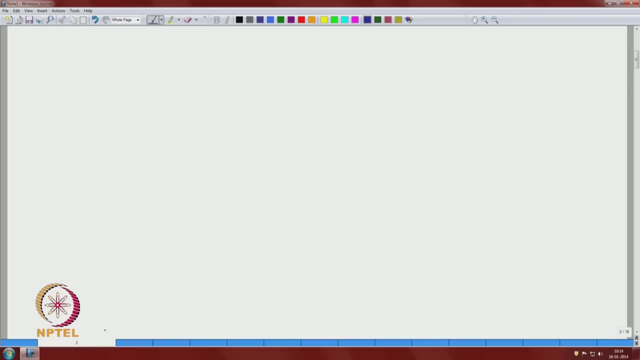 the plane x 1 x 2 moves in the x 1 x 2 plane. So what is happening here is that this can think it as a function of x 1 x 2.. This can think it as a motion of a particle in the plane x 1 x 2.. This plane x 1 x 2 plane. 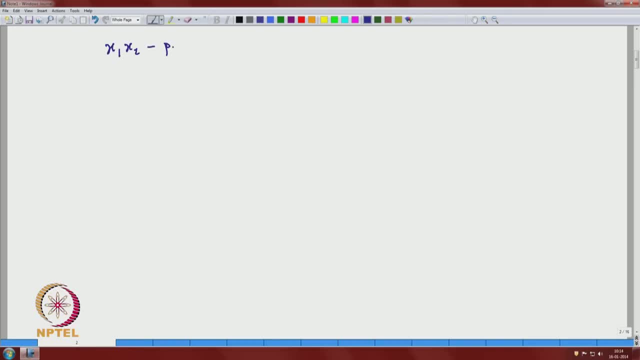 is the phase plane, called phase plane, associated to the system, associated to the system. So this is the phase plane. you see, And you want to understand us. This is the motion of the particle and x 1 t, x 2 t is the parametric representation, with the parameter being time. 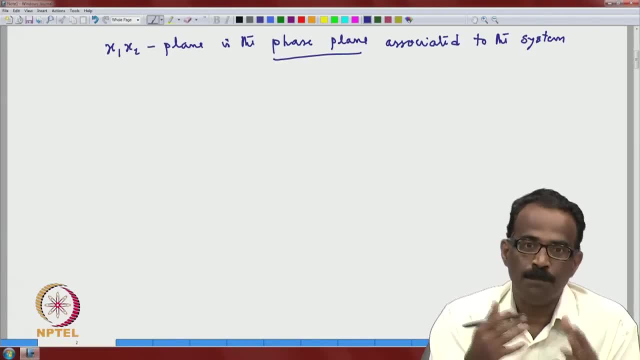 in the x 1 x 2 plane. So you want to see the picture, the trajectories in the x 1 x 2 plane. You see you have x 1 here and you have x 2 here, And then you want to see how. 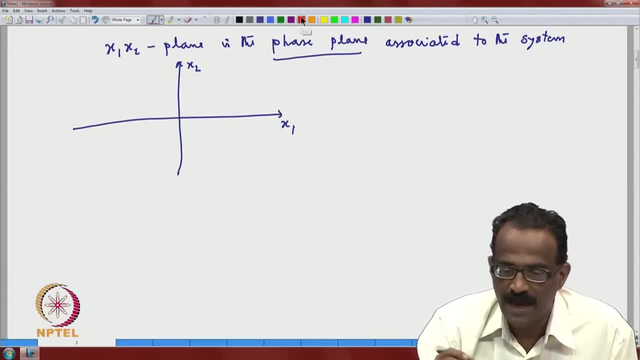 how the trajectories will move along. that If you look at, as you said, that A is an invertible matrix, in this case the origin 0,. this is the origin 0, 0 is the 0 equal to 0, 0 is. 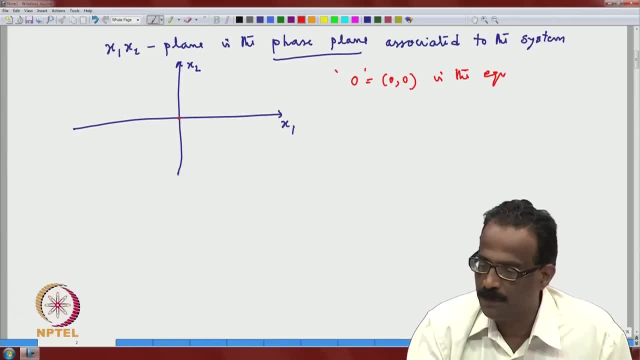 the equilibrium point is the equilibrium point which is a solution. So if any solution starting at the origin will remain there forever. But now look at the trajectories x 1 t which I have introduced for this. x 1 t is equal to e power t, x naught 1, and x 2 t is equal 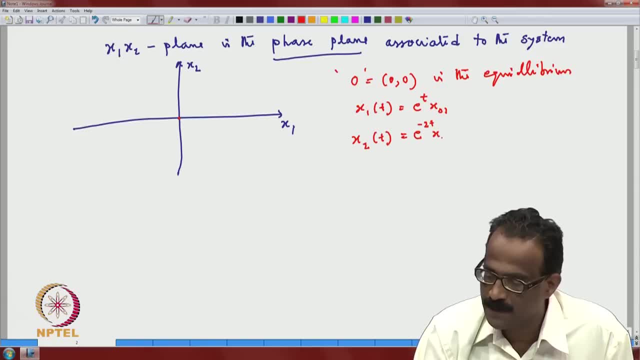 to e power minus 2, t, x, 0, 2, and this one, if you look at it, whatever be the x naught 1 or x 2.. So, depending on the sign of x naught 1,, this will go to plus or minus infinity, as t tends. 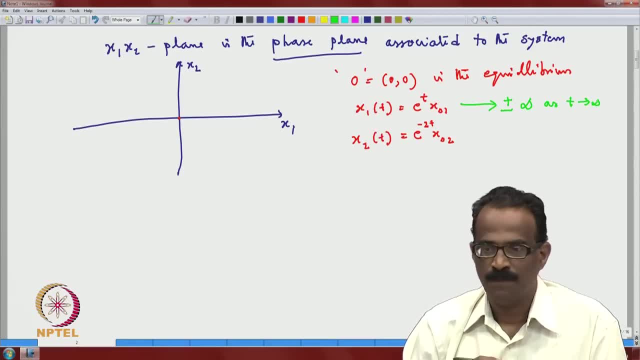 to infinity. On the other hand, irrespective of which coordinate it belongs to, this will go to 0, as t tends to infinity. So here is a situation: wherever be the initial point, the first component will go to. one of the component will go to plus or minus infinity. 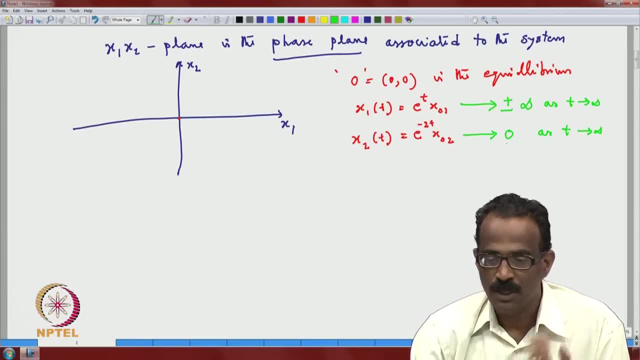 Or one of the component will go to plus or minus infinity and the other component will go to 0.. So you want to plot this graph in the x 1 x 2.. So what you do is that to plot this one, you eliminate this one, eliminate t. that is what you do it. you want a cross. 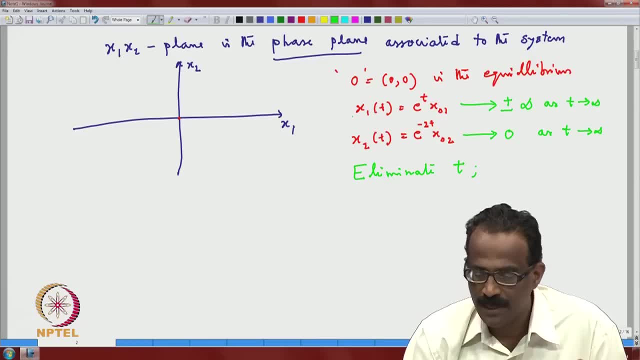 representation. If you eliminate here the best way to eliminate square x 1, so you will go back to that one. So if you square it x 1 square will be e power 2 t, but the e power minus 2 t, So you can put it under denominator. These are all will be constant. 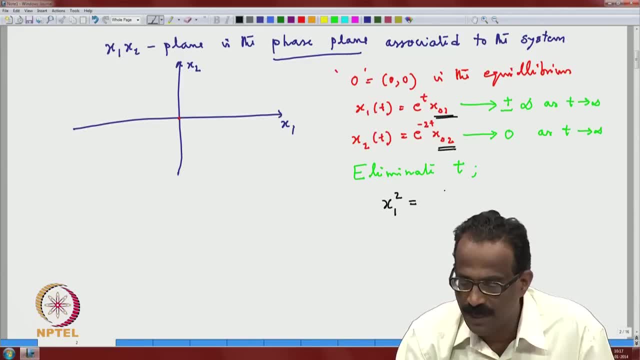 x naught 1 and x naught 2 will be constant. So you will get basically c by x 2.. So this is the closed form of this solution. So if you plot here, suppose you started a trajectory at this point, If you start that trajectory, so this is the point, nothing but some x naught. 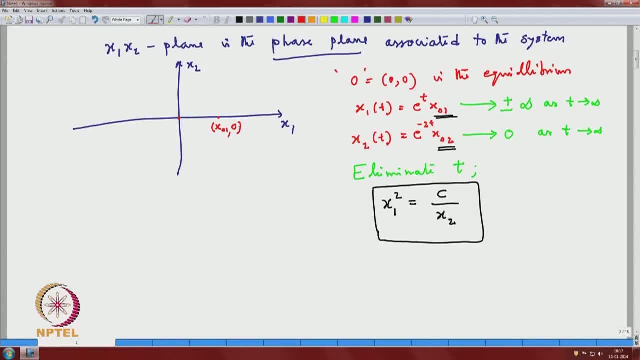 1, 0.. Since the second component is 0,. these are all these equations. is a decoupled system, x naught 2 will be 0.. The trajectory will remain. x 2 component will remain to be 0. 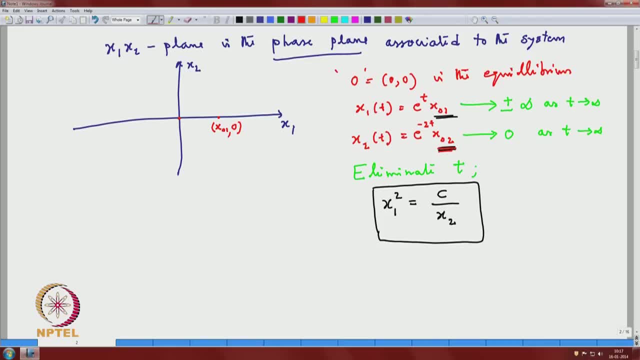 all the time. So the trajectory will be here, So this will be a trajectory basically. So this is the trajectory. On the other hand, if you start a point here, so this is also a trajectory. Only thing: which direction we will move, the direction of the motion is the only important thing you have. 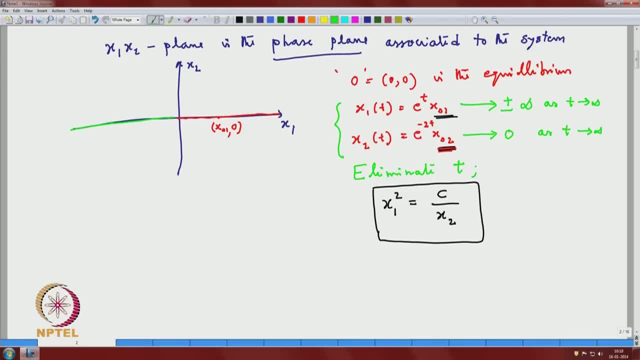 to see and the direction will prescribe whether it will go to plus or minus. So in this particular case, so if you start with a point here and, as x, 1 component will go to 0, infinity, the motion will be in this direction. 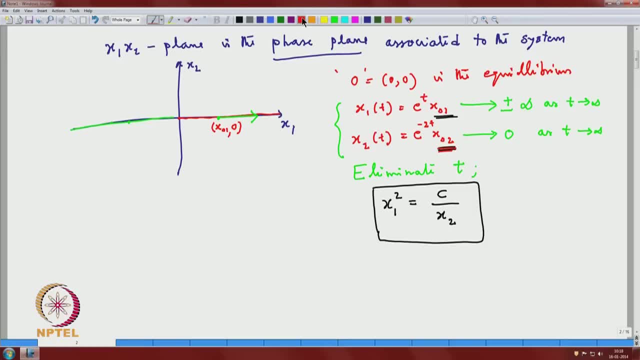 So if you start from here, the motion from, if you start from here, this will move in this direction. On the other hand, if you look at it here, if you start a trajectory from there, the again the trajectory will remain in the x 2 itself, because x 1 will. 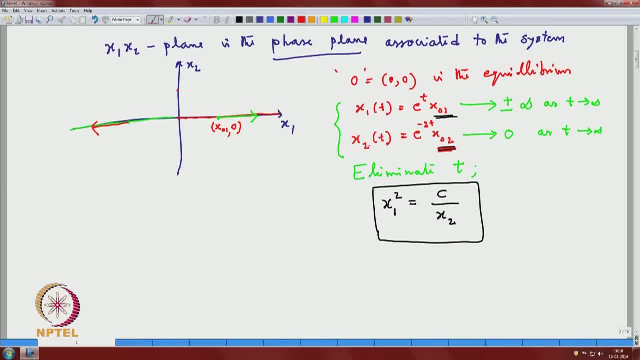 be 0 all the time, but the x 2 part is going to 0. So the trajectory will move towards here. If you start from here, the trajectory will move here. So this is, at the time, t equal to 0 or any other time, and as t this arrow represents, as t tends to infinity all the 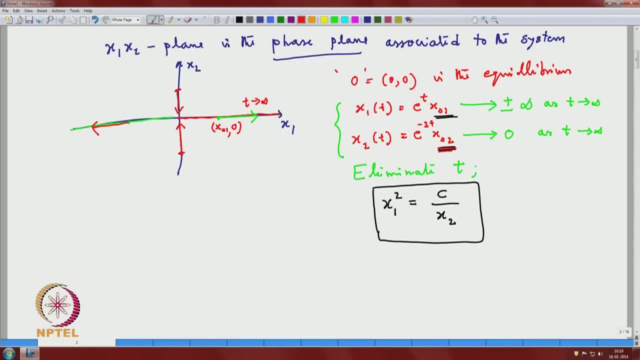 time. You have to understand this arrow as t. So if you move from here it will move along this direction to here, all that equilibrium point. but if you start from here it moves away from the equilibrium point. Now let us start from here. So suppose you take an. 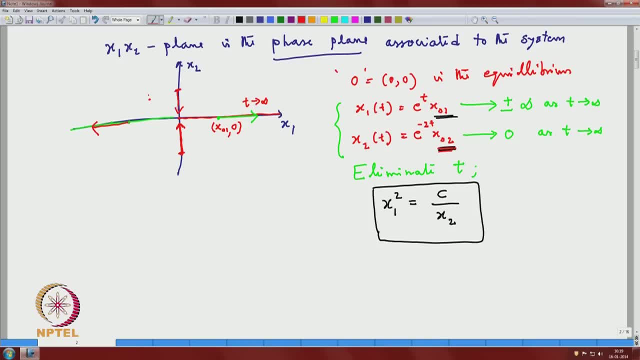 equilibrium point here. This is your point x naught. So if you start from there, your trajectory will the graph tells you is something like this kind of thing, is something like a x 1 square equal to x 2.. So it will the graph if you plot here. so this is a best. 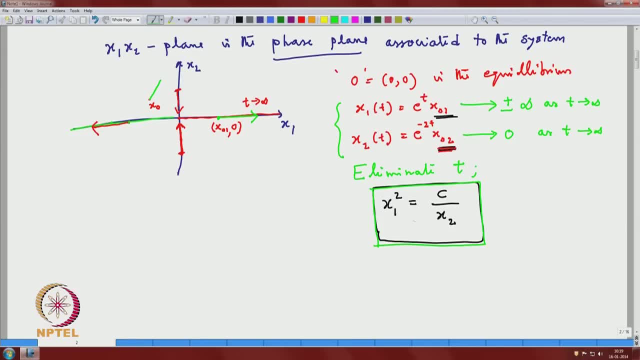 example to see. it will plot here your trajectories, if you plot, because this equation will be defined for not only for t positive, it defined for t negative as well. So if you start here, your trajectories will be here. So all your trajectories will plot here. So if you so, 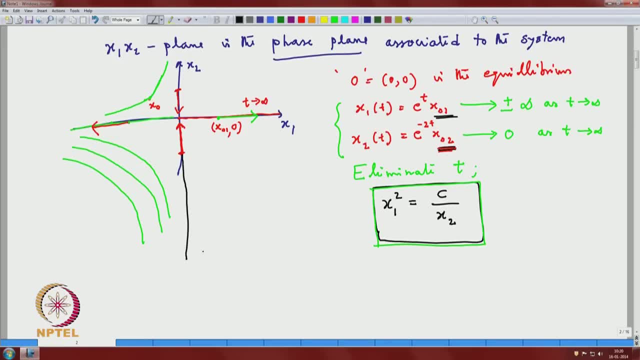 I have your thing. So if you have your trajectory, you have your trajectories. like this: If you have your thing, you will have your trajectories here. If you plot here your trajectory, all the trajectories will be here. So only thing. 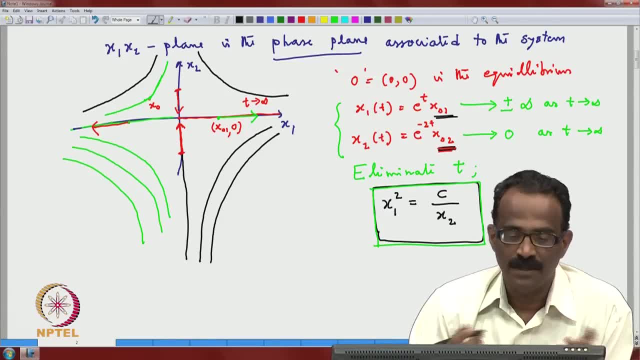 is that? where is the motion, in which direction this will move? For example, if you start from here, as you know, that x 1 coordinate go to infinity and x 2 coordinate will go to 0, as t tends to think, it moves along this direction because this is the one x 2 component. 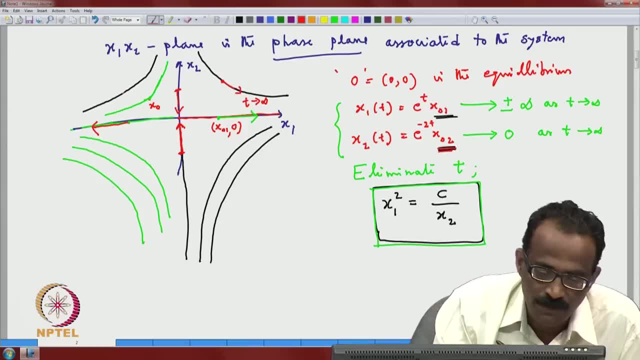 is going to 0, x, 1 component going to infinity. So if you start so it will match with this. It will move in this direction. if you start from here. So this is the part where t tends to greater than 0 part. So if you move here it will move in this direction. If you have 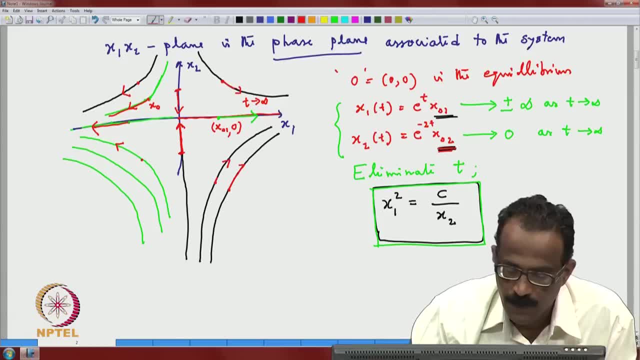 initial point. it will move. So everything moves away from that. So it is t. So the phase plane, together with all the trajectories, is the phase portrait of the system. So this is the phase portrait of the system. So this is the phase portrait of the system. So this 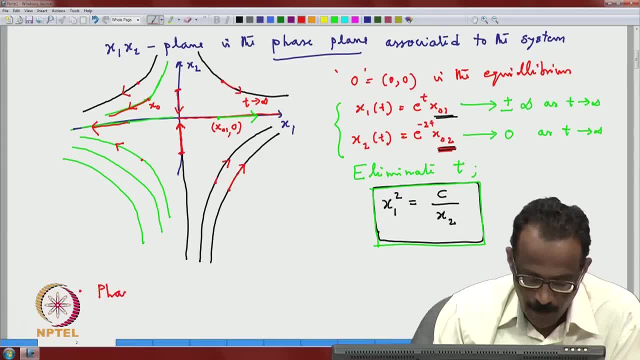 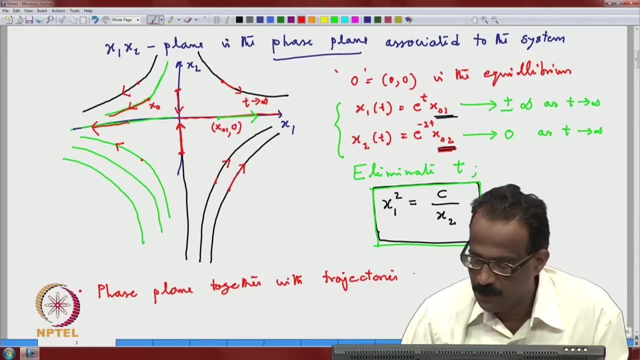 is the phase portrait of the system. So the phase plane, together with the trajectories, is called the phase portrait of the system, called the phase portrait of the system. So this is the phase portrait, phase portrait. It is a portrait, So this gives you the complete 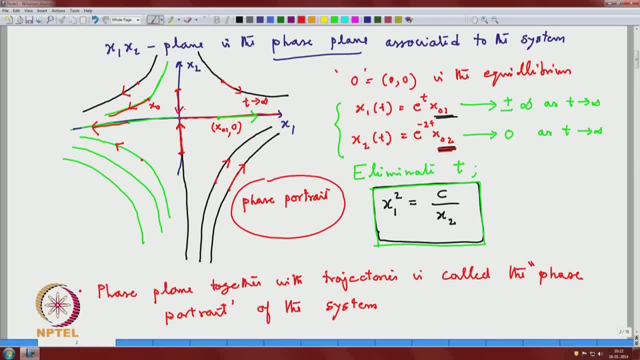 analysis of your trajectory and such an equilibrium point. So this equilibrium point because the trajectory, at least one component, moves. So if you started trajectory anywhere here it is moving away. As t tends to infinity, it moves away. You see, that is what. So move away from the equilibrium points, Whenever that happens. 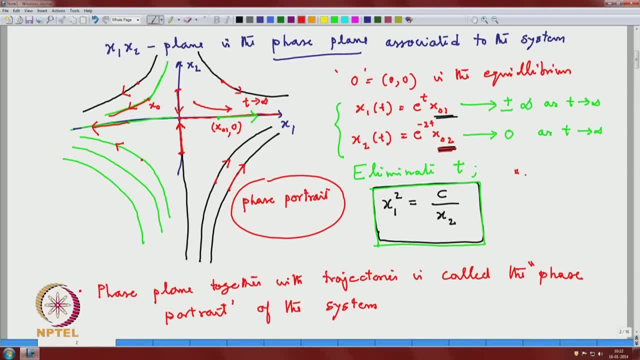 such things are called unstable. So this is an unstable equilibrium. It is not stable. So however close it is, it will eventually move away from that unstable equilibrium. So unstable equilibrium point In this particular thing. there are different types of stable. 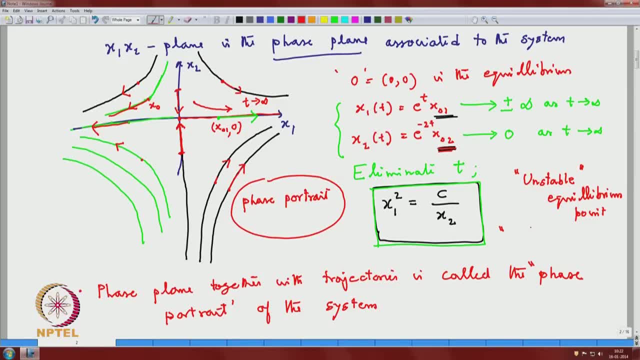 and unstable equilibrium. This is something like a saddle. You see, it is sitting, something like that. The trajectory is moving and it is called the saddle point. This equilibrium is a saddle point. See, this is the situation about the… So 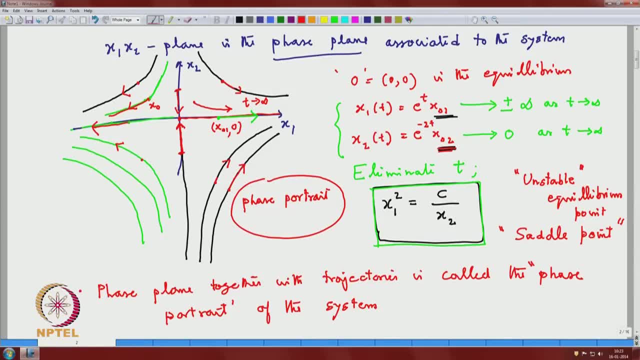 you have the phase plane where your trajectories are moving in R n space In n dimension. this phase plane is called the phase space For R 3, the phase space is x 1, x 2, x 3 phase and R 4 is a 4 dimensional phase plane. So if you are studying a system in n dimension, 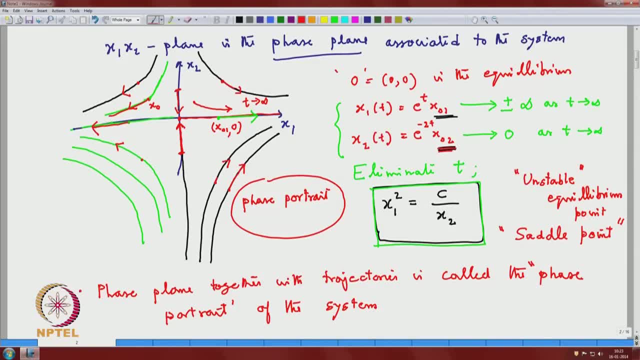 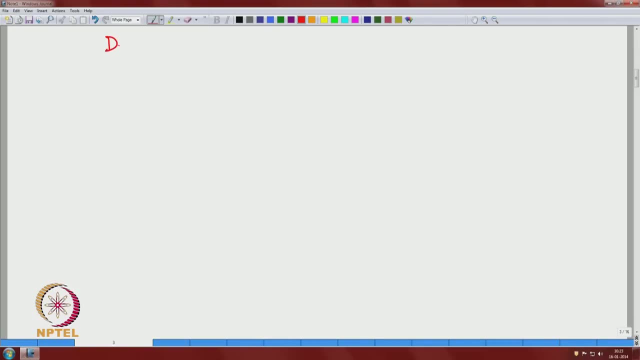 and it is. you want to see the motion of the trajectories in them and that is the corresponding phase portrait. So with that we have another notion called dynamical system. You can also call the given system to be dynamical system, but we can also give a more thing. Consider the map v. 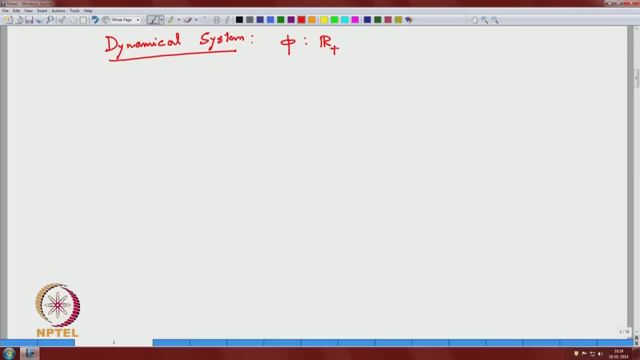 from r plus or r. If the solution x is r plus, cross r n to r. n given by phi at t and x naught is nothing but x t, x naught. So what is your system? x dot t is equal to a x t, So this is the. 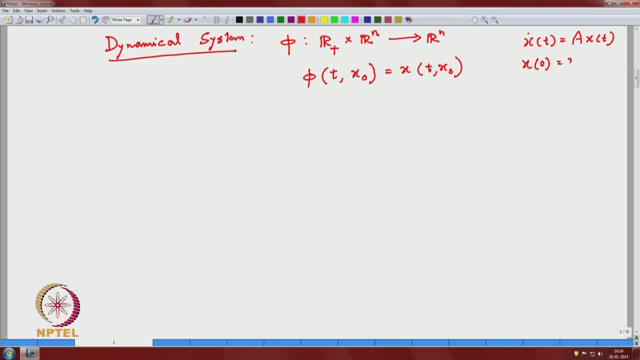 solution: Let us start with 0,. does not matter As far as this system is concerned whether you start with a t naught or start with a t, does not matter. So this is nothing but the solution at the time. t starting from the point x. So if you start in R n R, 2,, so 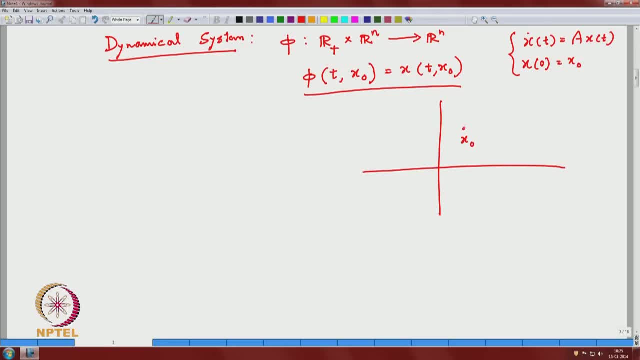 you will have an x dot here, The solution will move along. this last thing, and this is nothing but the. So you can imagine, the dynamical system is nothing but the motion of the particle. Once you fix x, naught, it is nothing but the motion of the particle. 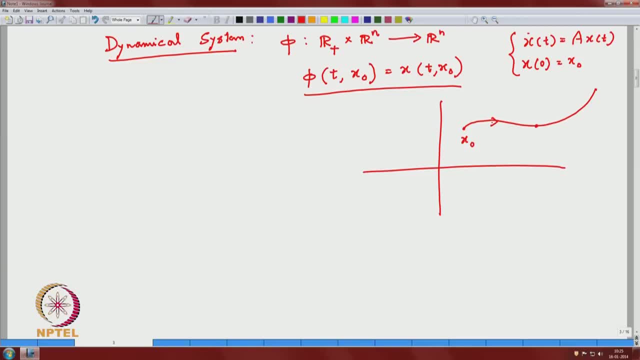 along a trajectory and it gives you the position of the trajectory at time t, starting from x naught at time 0. For this particular system, x dot t is equal to a x. t with x at 0 is equal to t, So it is a. in fact, it is the motion of the particle dynamical system is the motion of. 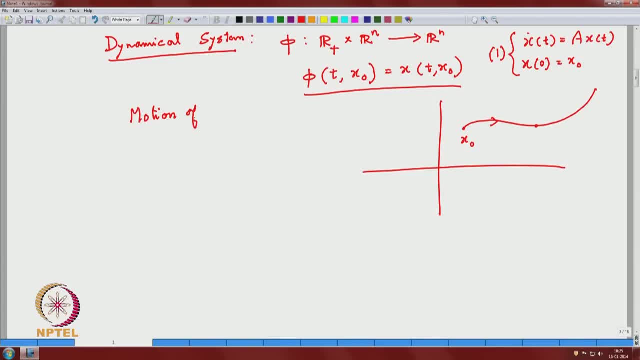 the particle in the phase plane. That is what you have to understand. This is an another related notion. This gives you a better feeling about this. What is called? that is what is called a flow of the system. Now, what you do is that we will have a physical 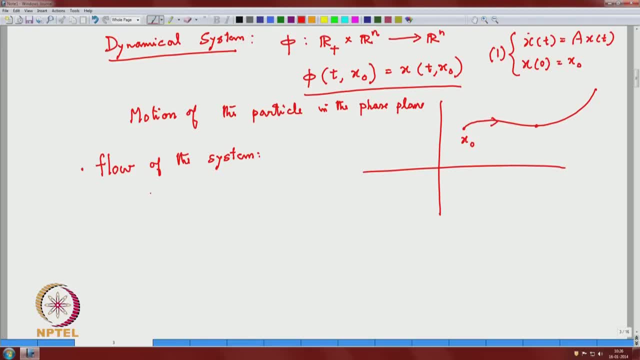 motivation for this. You look at fixed t. you consider phi t. phi t is that, namely e power a t t a, e power t a for this system. This is a mapping from R? n. you can view that this is a mapping from R? n to R? n for any dimension, So you collect everything. So 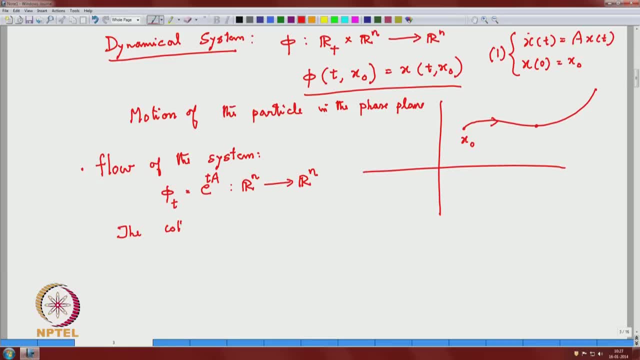 this collection is called the flow. actually, The collection phi, t is equal to e, power, a, t as mapping, T, a, such that for all t in the system you have, as you see that, not only for t, r plus you can consider- is called the flow of the system. What is the flow doing? What is the 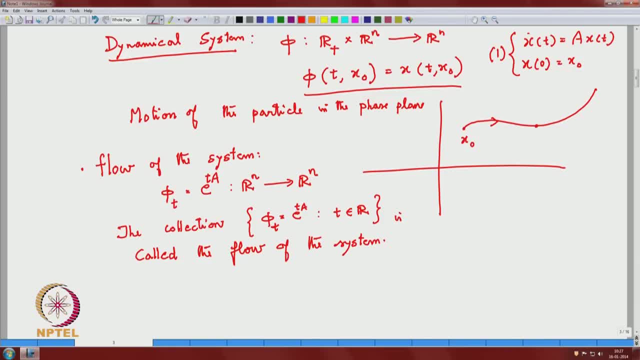 advantage of the flow. The flow here, for example, the main advantage. when we look at it, a fluid flow, you can think that a fluid at time t equal to 0 in one position. Then you view the fluid as particles and then for each particle, after some time the particle will be at another. 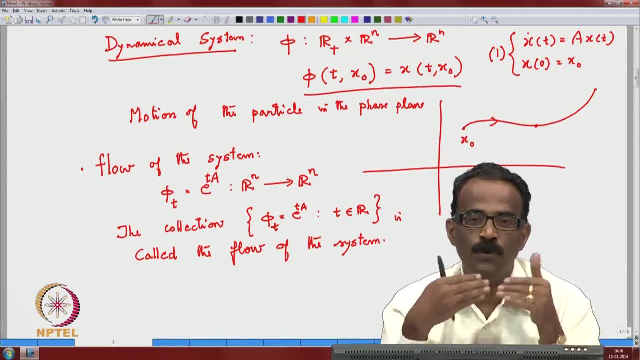 point. But this does not give you this view of a motion of the particle. If you view at least a particle in the fluid, for every particle it moves to some other position at at sometime. t but for a layman point of view or a natural point of view, When you 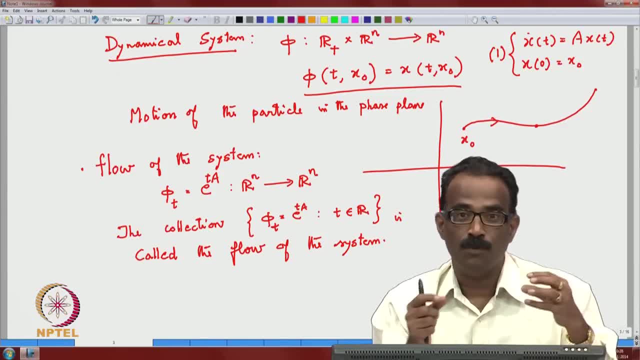 look at a flow. we never see the flow as particles are moving. Rather we see a collective motion of particles. So this forces you to understand the motion of just one point. We want to see that both motion of point are together with its neighborhood. 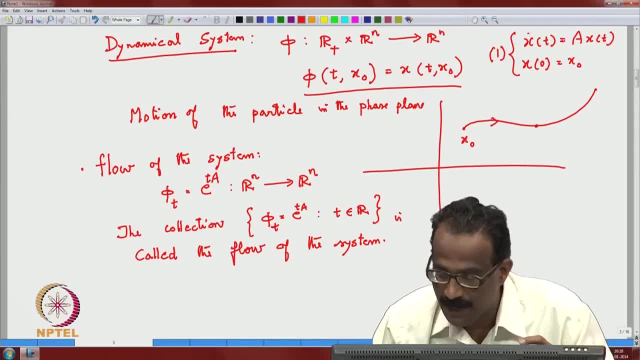 In such a zaman where the motion is Kanma Thiragam pública, So you can match the motion plot and certain thing의 in his neighborhood. So if you start with at x naught, this is at different v x naught and look at this neighborhood. 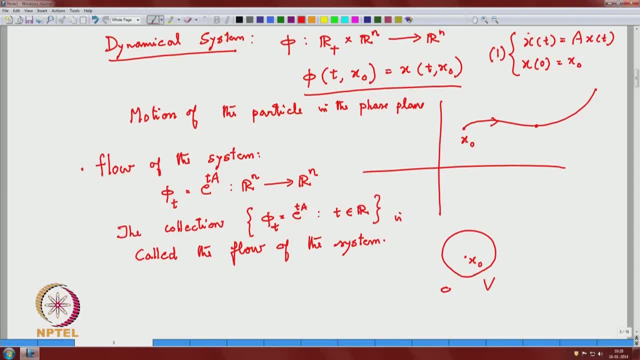 some neighborhood v and this is nothing but at the position phi at 0. So phi at 0 of v is v. that is because t 0 it moves there. Then for each t, for look at all the particle in the neighborhood and you collectively try to see this will be moving here and this 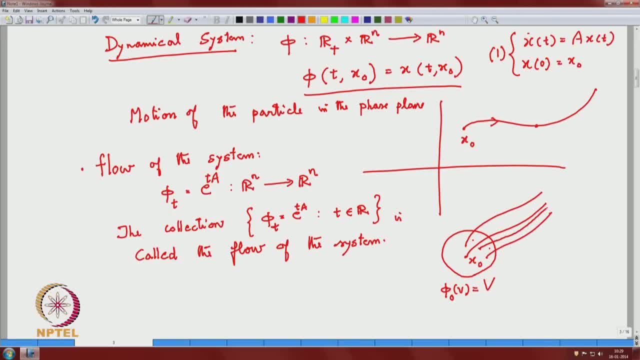 will be moving. here will be moving something. So you want to see this motion and all this will be at the different positions. This may be at a position somewhere here and you will get a neighborhood. So this is nothing but your phi t at v. So if you look at that, not 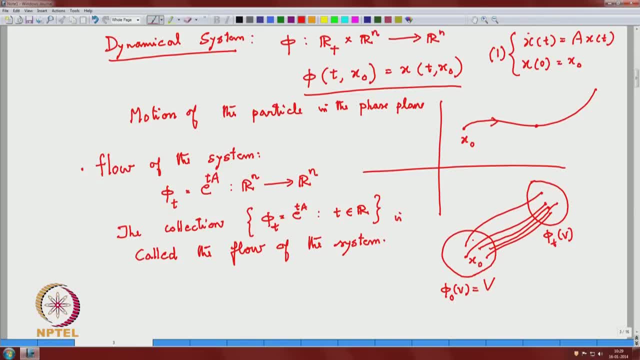 only the point x naught and all the neighborhood. you try to see the how the neighborhood together moves and that gives you the better feeling of the motion of the particles. So that is actually what you are doing: trying to do that through the flow of the system. 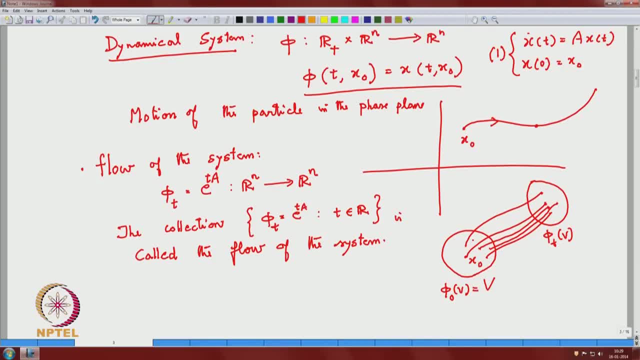 You see that a column or a neighborhood of the fluid moves in that direction. So that is what the flow gives you. the concept of flow and flow has some nice advantages, like kind of semi group properties and all that which you may probably learn in some other. 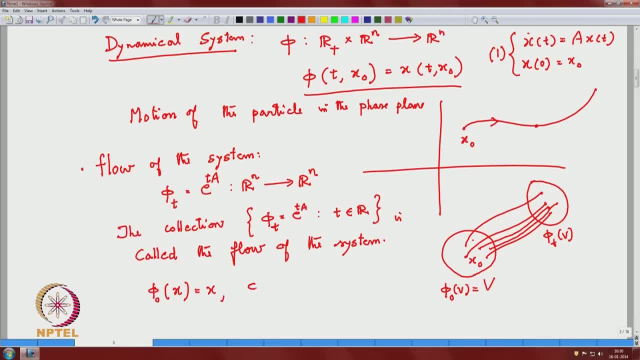 thing, Phi naught of x is always x. The more important thing is that suppose flow move at a time, flow from x. This is essentially tells you that the flow from x, phi, t of x gives you from the position x it moves to the position t at thing and then compose. 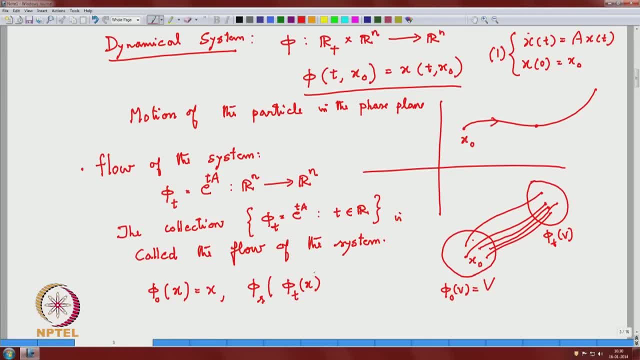 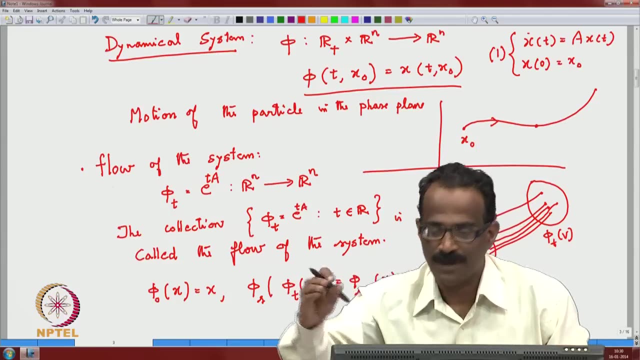 it with that phi of t will be the same as phi composition s plus t of x. This is a very important thing. So you flow moves from one position to another, another position, and then it moves is the same as flow moving from to other position. 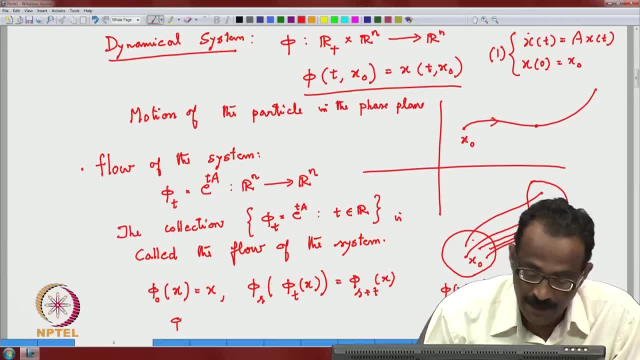 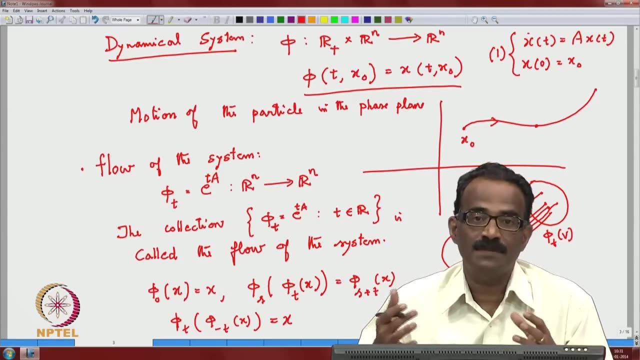 And another interesting property. this also has a group structure. in fact, for this particular system you will have phi, t of phi minus t of x is equal to x. In general, many of the flow, if the reversible systems, you may not get the last property, but for this systems, 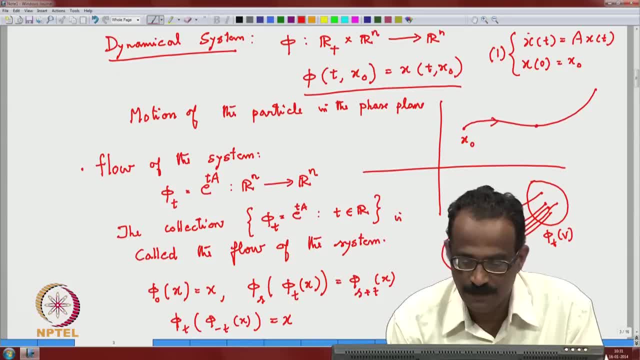 are. So you can also reverse the flow. that is why it exist for all t in R, but in a semi group. when you go to partial differential equations, etcetera, when you try to understand this kind of motions, you may not get a group structure, you may only get a semi group structure. 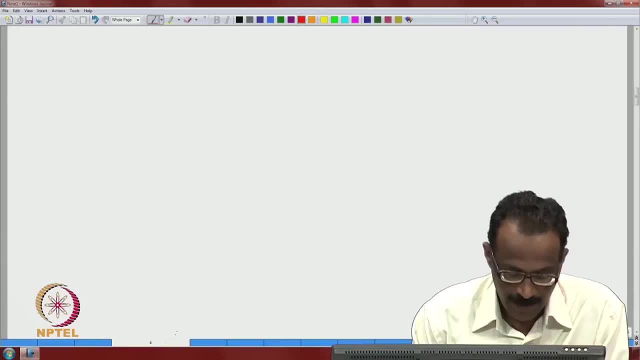 that is anyway not the topic of discussion here. And one more notion which you probably would like to think. so these are all some geometric way of understanding Vector field. so to understand the thing is not as you see now, is not only understanding the solution, how to interpret the solution, how to view the solution, all part of the study. 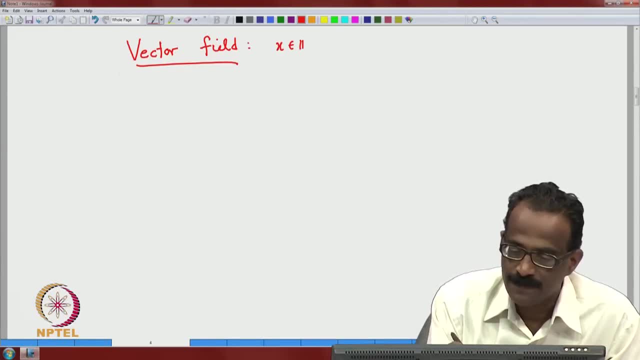 Vector field for given x in R n. A x is another point in R n, but in the beginning of our discussion long back In the previous lectures, We said in R? n you can view either the points of R? n as points or you can view also a point. 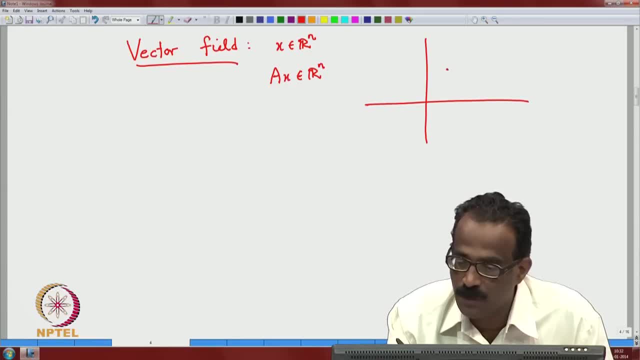 as a vector, just like we have seen. So either you can view this point x or you can view that point as a vector here. The advantage of this vector: you view this as a vector. I can put this vector with the same length parallel to that so you can get that view. 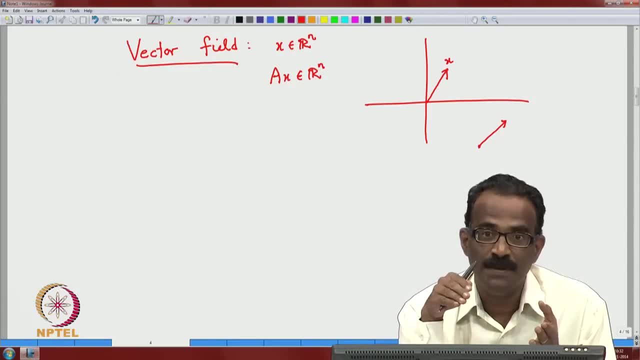 So, for example, when you have a fluid flow of a particle, The position of the particle, The position of the particle, The position of the particle, you like to view it as a particle, but on the other hand the velocity at that point is also a point in R, n, but then is better to view the velocity? 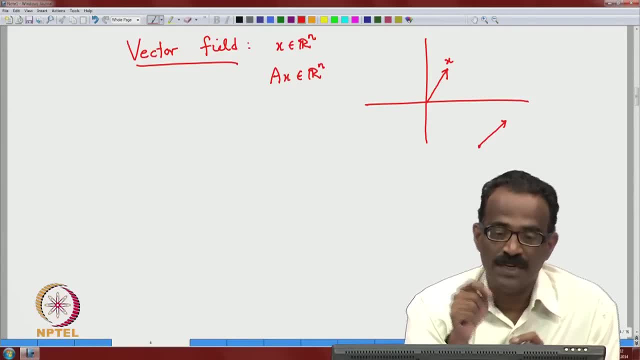 is a vector placed at that point. So when you given a dynamical system, x dot is equal to A, x, x, t, you view it as a position and A- x you view it as a vector. So that way any matrix A, any matrix A, gives a vector. field structure in R, n gives a vector. 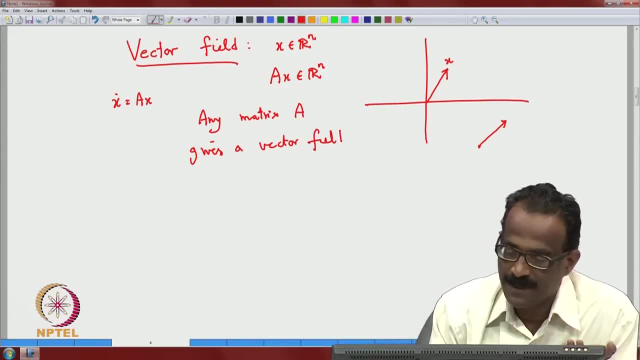 field structure: vector: field in R n. So what you can saying is that for all the points here x, you have a point here x, you can associate a vector. This is vector is nothing but A, x. If you take another point, you will have another vector. all the points can be associated with. 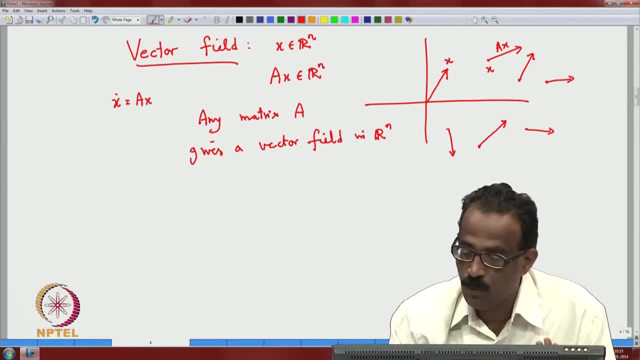 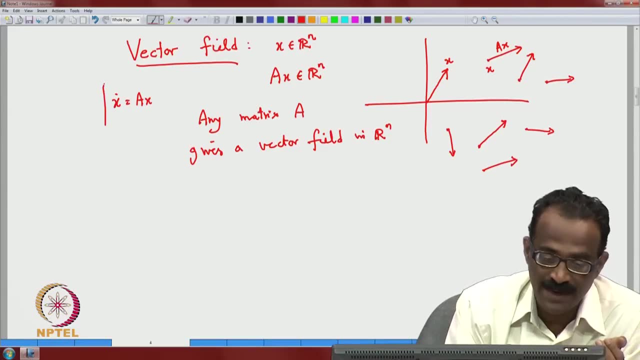 vectors, So want to know for a given dynamical system. so if you so, if you look at it here clearly, what are we trying to? we are trying to associate x dot equal to A x. so when you are looking for a solution, 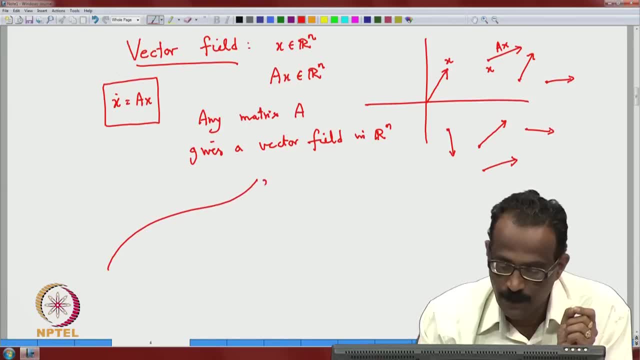 x dot equal to A x. So we are looking at this x t to this dynamical system: x dot equal to A x. you are looking for this trajectory: A x, so that x dot is equal to nothing but your tangential vector field. this tangential vector field should be A x. 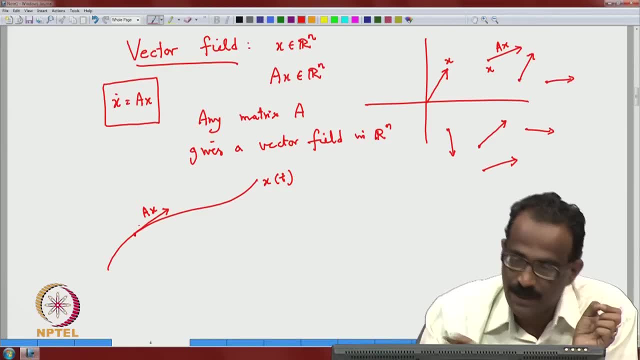 So the vector associated to this point, each point, should be A x. So A x should be A x each point. So we are looking at a trajectory solution associated to that one. you want it. these are all should be your A x, you see. So that way, a solution, a trajectory. 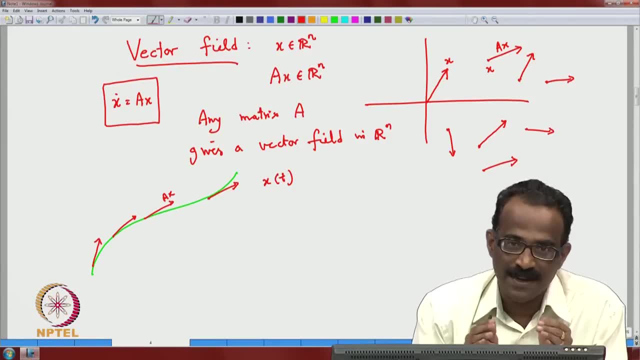 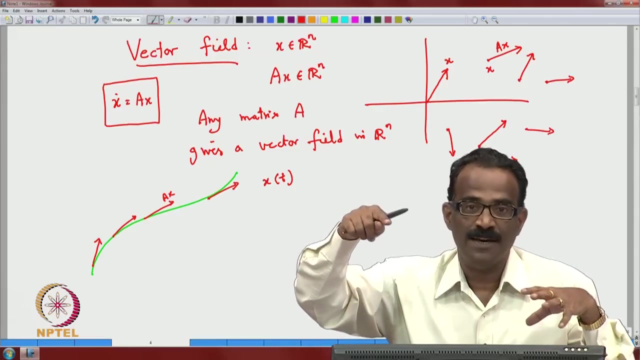 x, t is a curve. x, t is a trajectory to the solution. at each point the tangent is given from the vector field. The moment A is given to you, you have a vector field. given a vectors are associated with all R, n. So you are trying to find trajectories in such a way so that 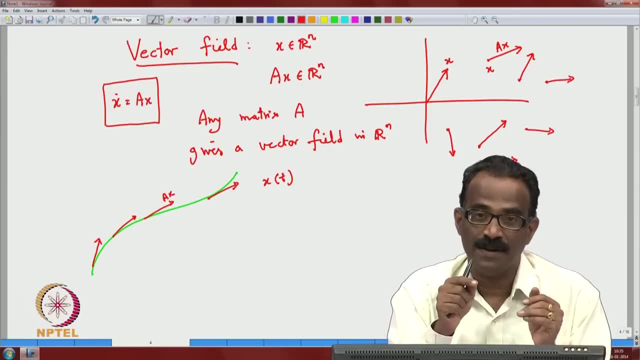 each point on that curve, the trajectory. the trajectory is given from the vector field. The tangential vector coincides with the vector field given to you. So the moment you are given a linear system like A x, x dot equal to A x, you want to plot your vector field. 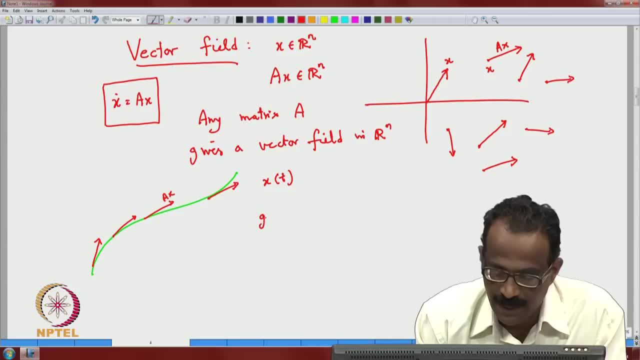 in that way. So for the given example, given example earlier, given example earlier. so if you try to plot your vector field, you can see that the vector field, you already know the trajectory. So your vector field will be like this. So if you plot your vector field, it will. 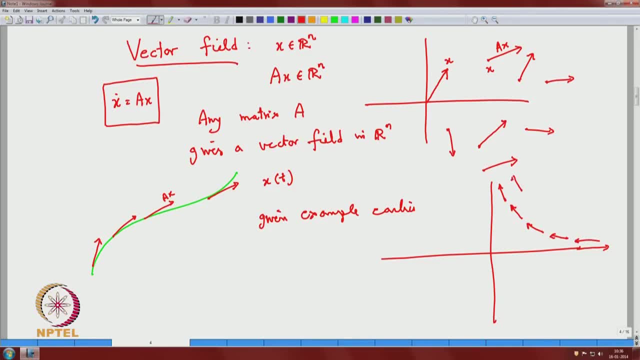 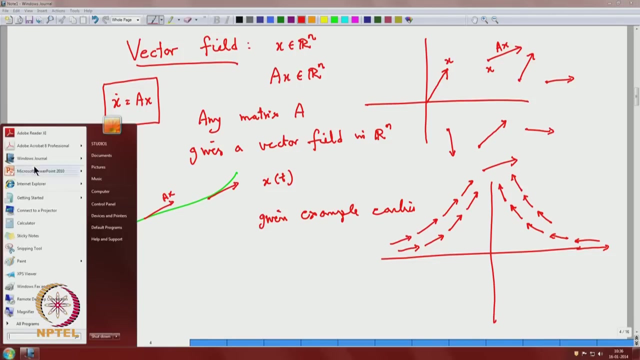 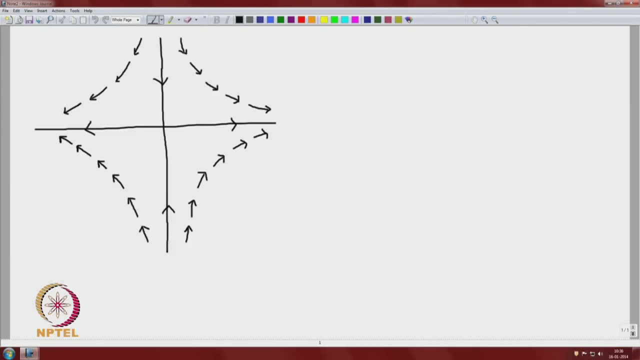 be something like that. So if you, so you get all your vector field like this: This is your vector field associated. So if you plot it here, you see, So we will plot it here. So so that is the vector field. let me plot again the vector field. So if you, 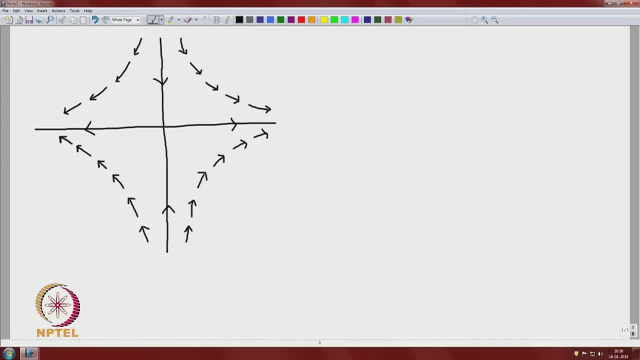 have your vector field to that example and something like that: This is for the given, given example. so it may vary like that: If you plot from here, that is how curves. Similarly, if you plot here like that, this point, this is the vector field, No, these directions. 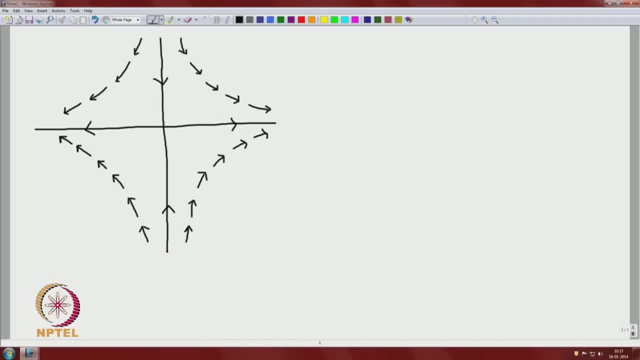 have changed. That is not the direction. So the direction is in this direction. So if you plot here, the direction will be like this: If you plot here, this will be the direction You get each point, you will have the corresponding. this will be here because it is a stable one. 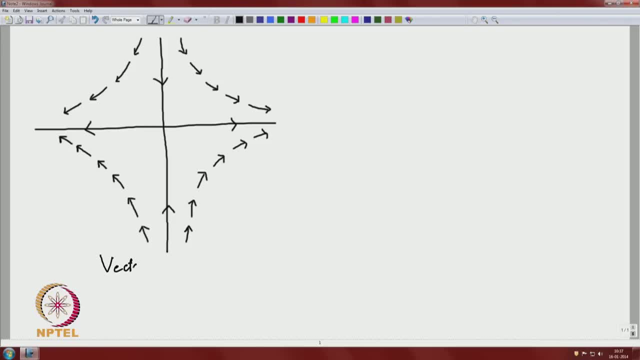 So this is the vector field. So every system you will have a vector field associated with that. So what I would like those who are learning here as an exercise, plot these things. Exercise: plot the curves. plot the curves and vector fields. curves and vector fields. 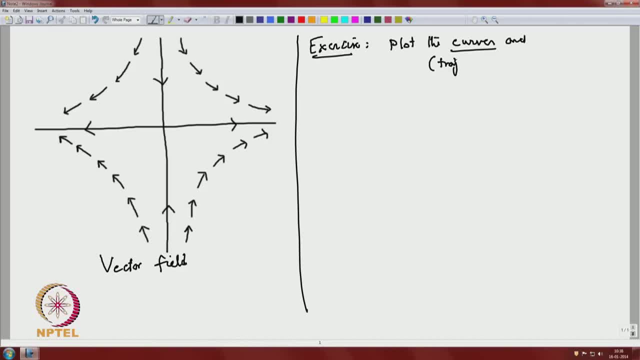 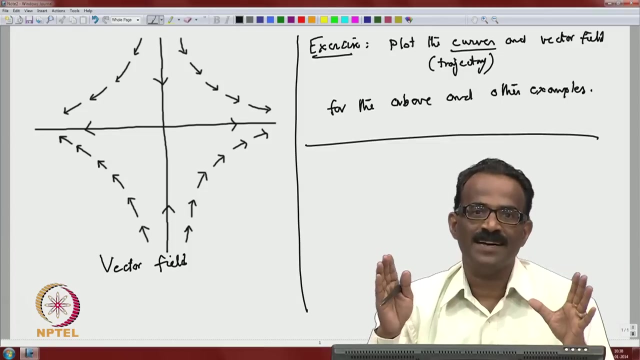 Curves means solution trajectory. I mean trajectory and vector field for the above and other examples. So what we have seen is that when you have the solution trajectories, if you plot all the tangent vectors, you will get your vector field. On the other hand, 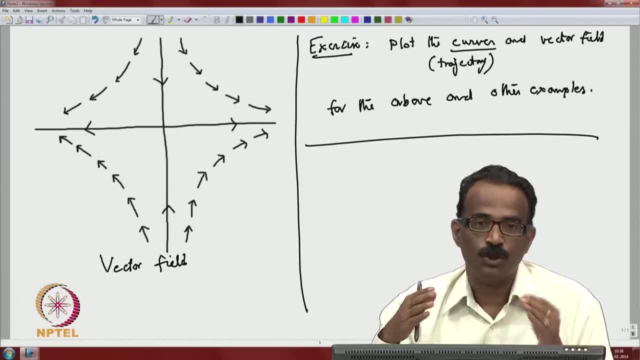 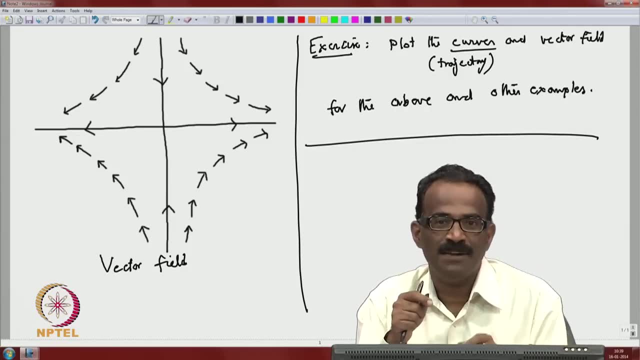 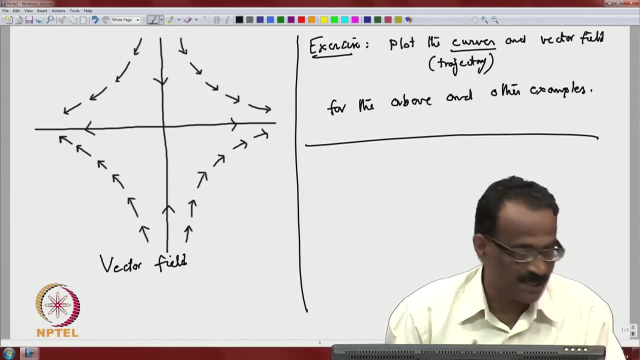 if the vector field is given, you take any trajectory so that the tangent vector to that curve should be from the vector field. It will be a vector field associated to that and that curve will be the solution to the system. With this basic notions, we will see. 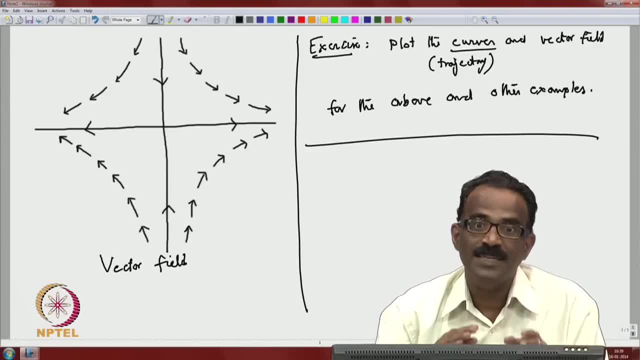 more and more examples as we go along. What we have seen is only a saddle point example. Now we are going to see the Ender analysis for the two by two systems, which we will do that. So basically, we want. 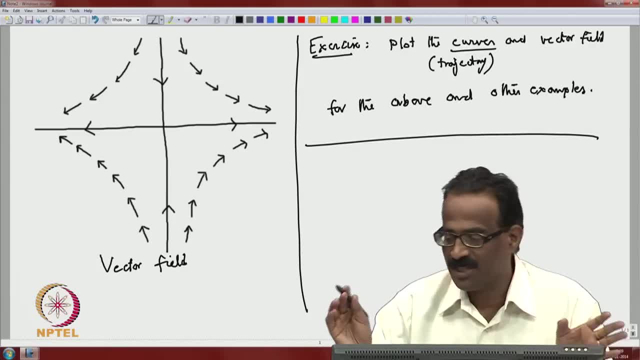 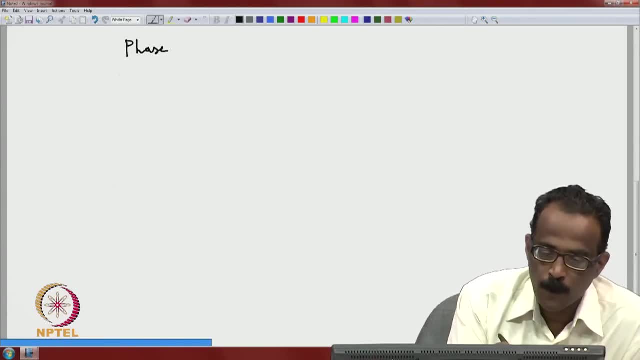 to do a phase plane analysis of two-dimensional system. That is what we are going to do now: Phase plane analysis, analysis of two by two systems. So you have some terminologies of phase plane and you are going to see- not only here- even the other module of non-linear 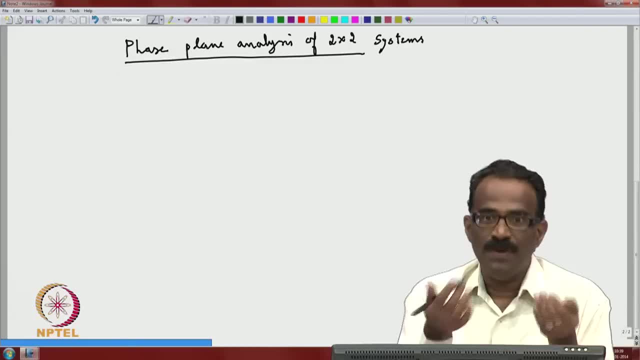 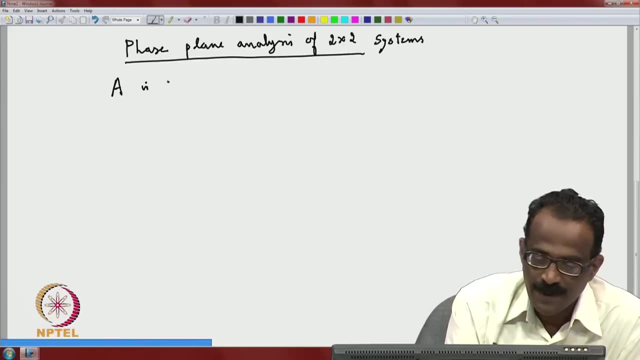 systems. So what are the things Now we have to recall from the linear algebra? We want to know if a is 2 by 2, we want to know what are the possible 2 by 2 linear equivalent matrices. Typically this can be classified into two. 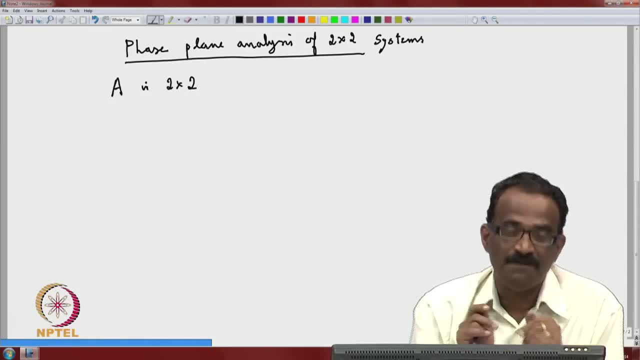 What are the possible? two by two linear equivalent matrices. Typically, this can be classified into three different categories. What I am trying to say that the linear algebra tells you that every 2 by 2 matrix is linearly equivalent to one of the three categories. 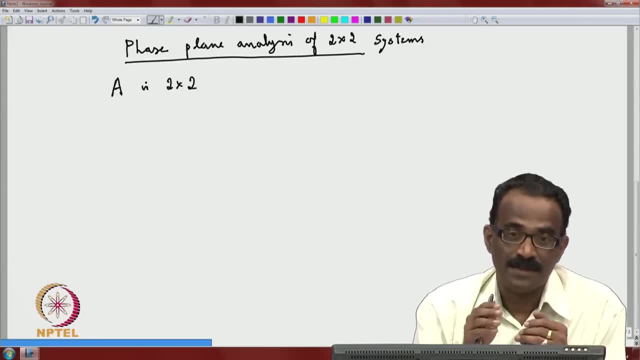 according to the existence, according to the Eigen values, whether it is a real Eigen value and distinct. It is a real Eigen value, but multiple real, coinciding Eigen value or the Eigen values are complex. So I am going to write the three things which I will not do. it Probably some of 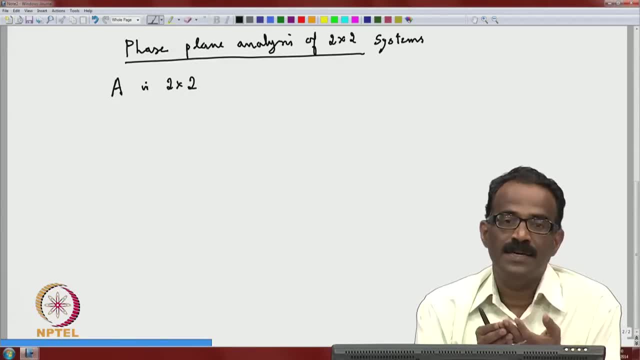 them. you will learnt in the basics. So that is what we called. So the type 1, we want to call it Type 1, in this case, a will be. let me put a notation: This is for linear. 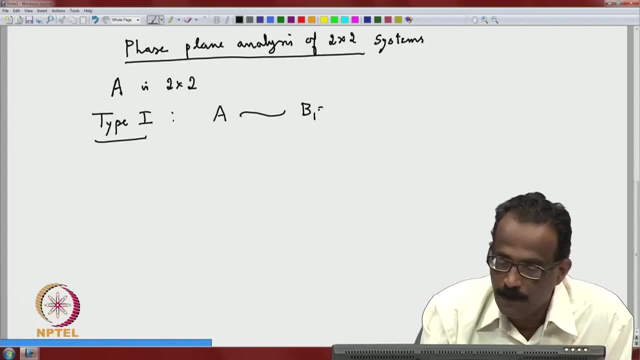 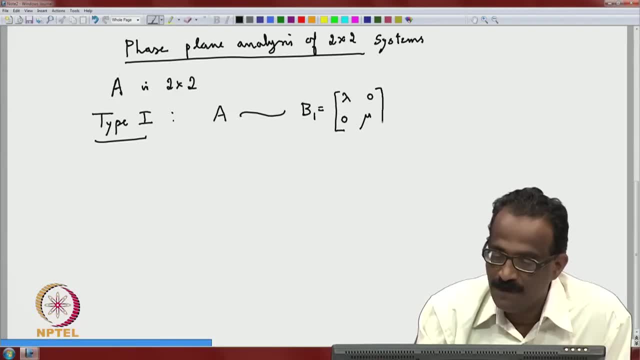 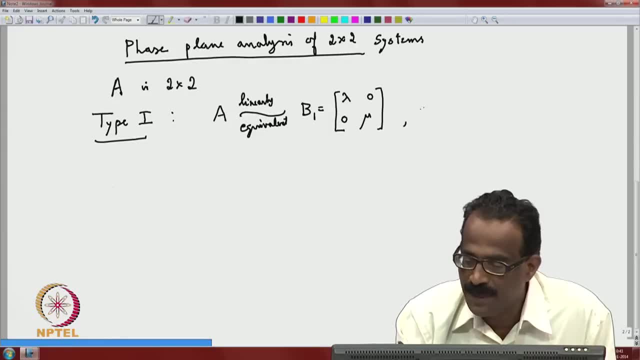 be written as p inverse of t. What is that means? your b 1 is of the form p inverse of a. p for some invertible matrix …. That is the meaning of a eigen. When is this happen? This happens when a has two distinct. 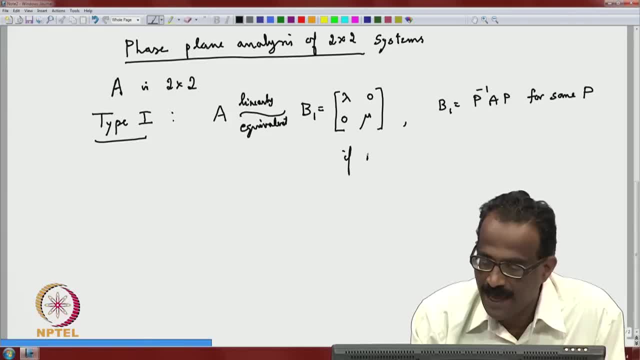 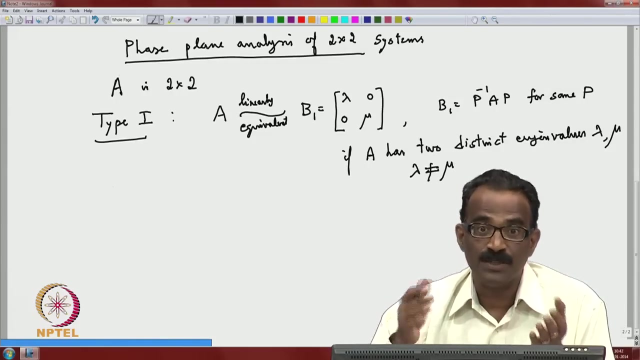 real eigen values. If a has two distinct eigen values, eigen values lambda min, that means lambda, not equal to min. This is the type 1 matrix. And what are the matrix of p? In this case, it is easy You look for, since there are two distinct eigen values it has. 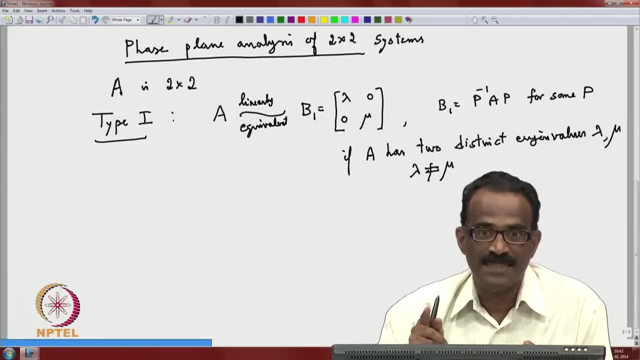 two eigen vectors which are independent. Put that eigen vectors as column vectors of p, You get your this thing. So p also can be constructed by obtaining the eigen vectors corresponding to lambda n mu. Because it is independent, it is invertible. 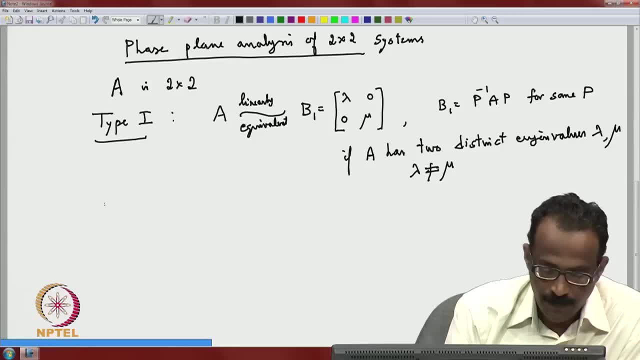 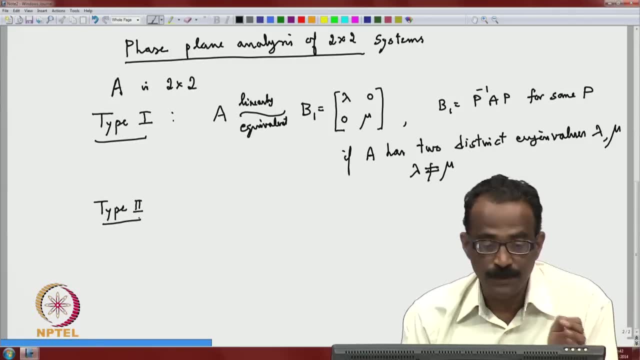 So that is the case. type 1 situation. So what is type 2?? Type 2, a will be linearly. There are two cases in type 2. also, It can be of this form: lambda 0, 0, lambda There. 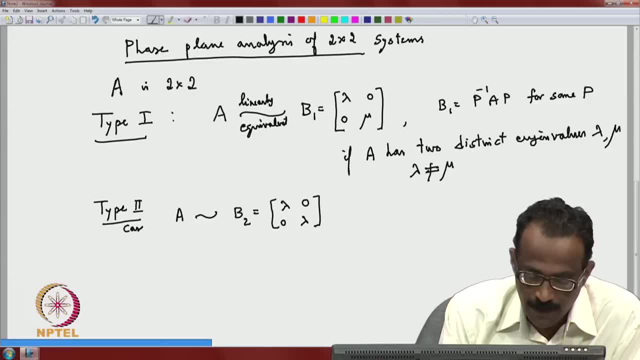 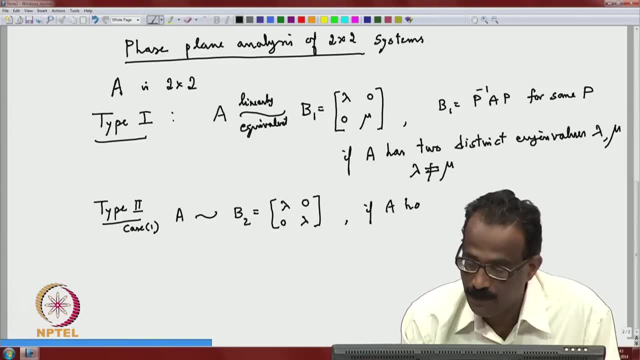 are two cases. So in type 2, there is a case 1. And this happens if a has a double eigen value. Double eigen value means eigen value with multiplicity, algebraic multiplicity- to double eigen value 2. That is the meaning. 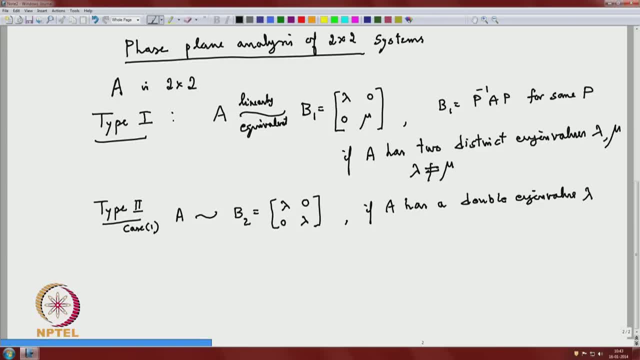 of double eigen value means eigen value with algebraic multiplicity to with. that is the thing. Now, when has an eigen value a coinciding value? there are two cases. there can be two still. it can have two independent Eigen vectors or it can have only one independent Eigen vector. So that is the problem. when you 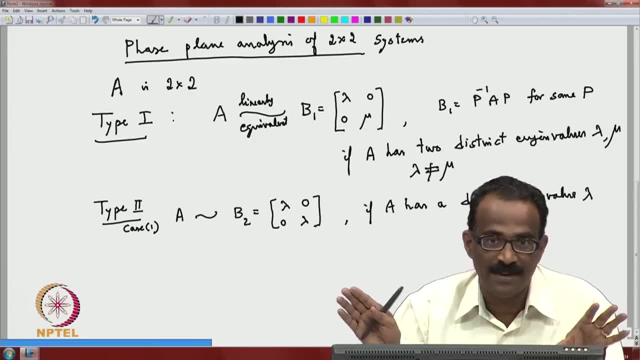 have two distinct Eigen values. you have two distinct independent Eigen vector. when it is a coinciding Eigen value, it is depending on the matrix. it can have two independent Eigen vector and that is refers to as the geometric multiplicity. So the classification. 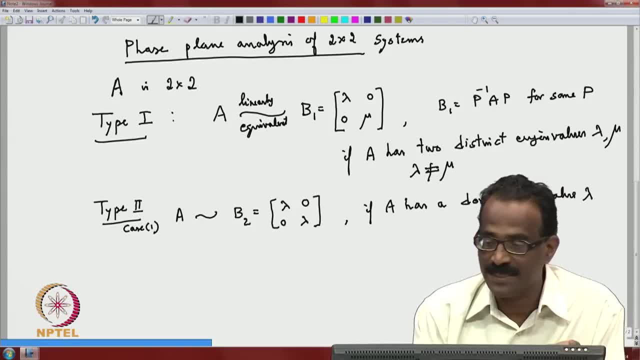 within. this comes because of the geometric multiplicity. So this is the case where it gives you two independent Eigen values, if it has two independent Eigen values and still it form a basis and you have the diagonalizability, and with two independent, with two independent. 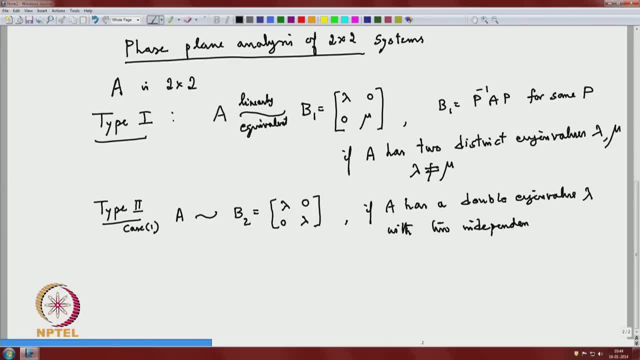 Eigen Eigen vectors, Then this will be equivalent to b 3. In that case b 3 takes the form a non diagonalizable matrix. The diagonalizability in general is not possible. 0- lambda- lambda Again. double Eigen value with algebraic multi Eigen value. lambda, but only one incoherent expression. 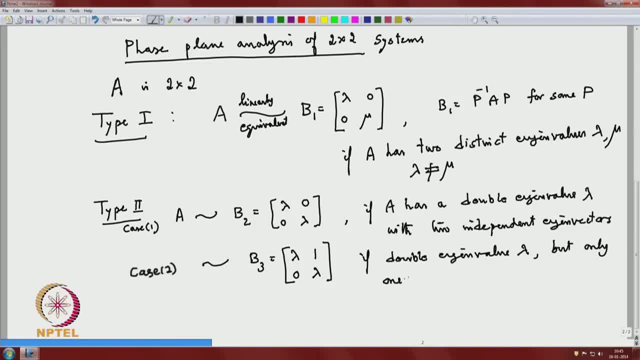 right independent Eigen vector. You see, the whole trouble in diagonalizability is the lack of independent Eigen vectors. That means- this is the first case- you have algebraic multiplicity 2, geometric multiplicity 2.. In the second case, algebraic multiplicity 2, but the geometric 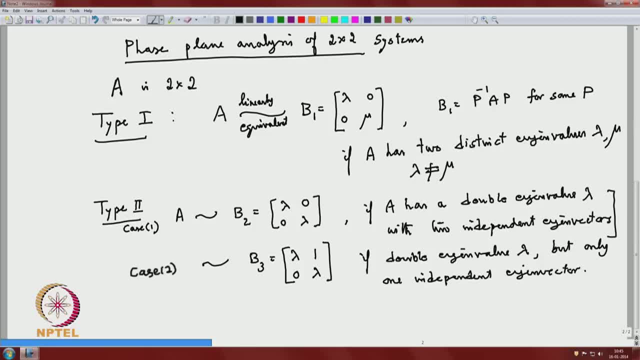 multiplicity is 1.. Hence it will give only one column vector for p. The remaining vector one has to construct to find the equivalence You want to write. a is equal to 2, you have to find p all the time In the other cases, getting p through Eigen vectors So that 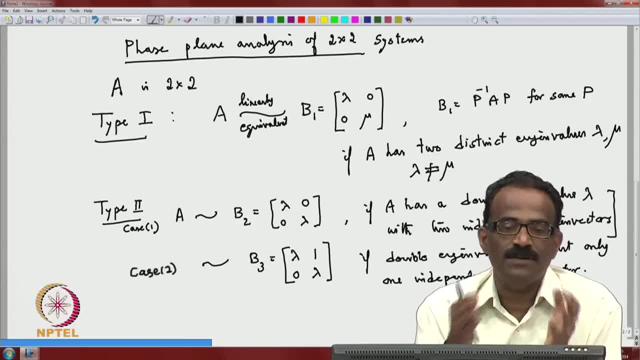 is the concept of generalized Eigen vector and that is the kind of the whole linear algebra and the Jordan decomposition theorem In higher dimension. there will be many complications. Some of the Eigen values are real, some are not, Some are complex, some are multiplicity. Certain things are simple Eigen value. So all complications. 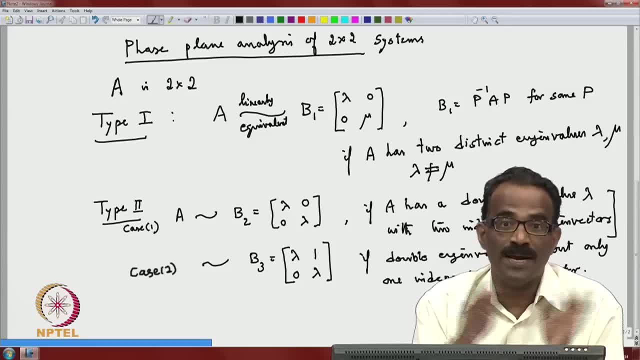 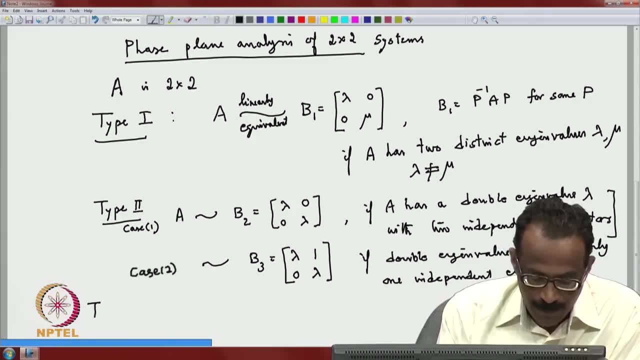 happen. So you have to distinguish all that. That is why you do not get the full diagonalizability, You get block diagonalizability. Type 3 is the last case which you know already. Now you know type 3.. 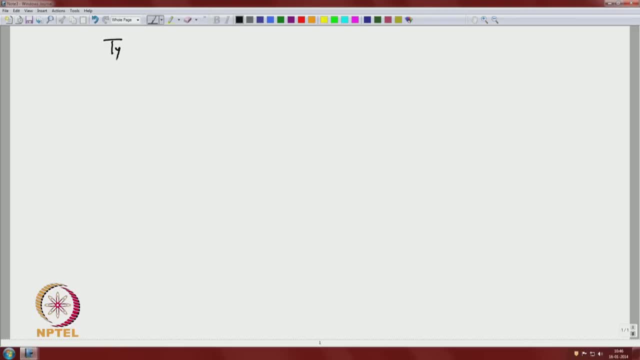 So the type 3.. This is the case. In this case, a will be linearly equivalent to a minus b, b, a, where a has complex Eigen values, Complex Eigen values. So a has complex Eigen values. Lambda is equal to a plus i, b and the other Eigen value, lambda bar, is equal to a minus. 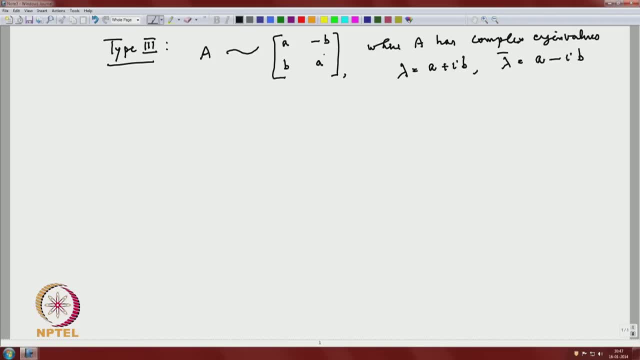 i b. So you have two Eigen values. So a will be linearly equivalent to a minus b, b a and this let me call it b four. So our aim now. So, if you want, as I said again, in again, if you want to understand, 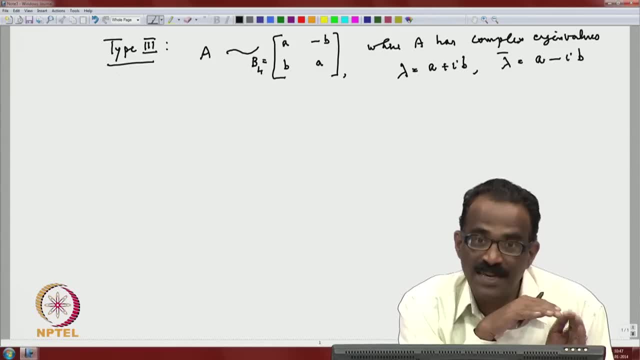 the linear system- x dot, x, x dot equal to a x, especially the nature and the behavior of solutions. it is enough to understand the systems corresponding to b 1,, b 2,, b 3,, b 4, and then we can recall. 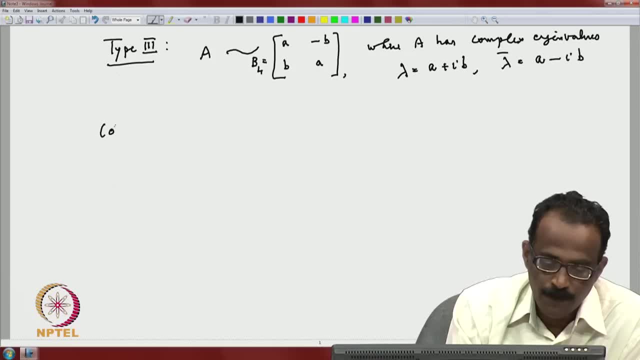 everything. Therefore, in conclusion, we only need to study the systems y dot. So y dot equal to b corresponding to each of these four b i's, b, i of y, where for all i equal to 1,, 2,, 3,, 4, with some initial values. say, y at 0 is equal to y. naught Once. 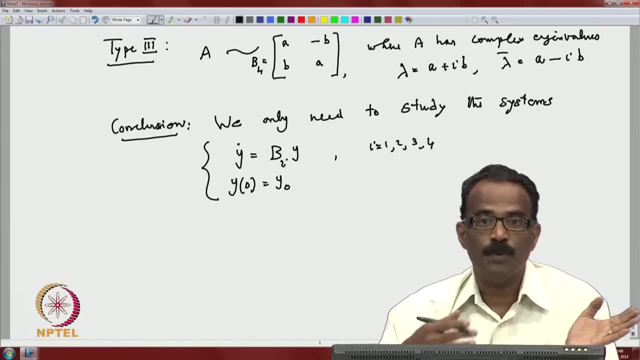 we know that we understand the nature and the corresponding a will have the same nature of that one, and then there will be a coordinate change, which we will see later, How these things are happening. So we are going to study this one by one now. So we 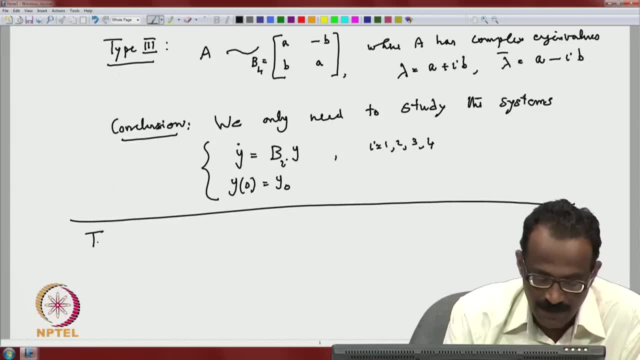 are going to do type I case. now We start with the type I. So in type i a will be- let me recall again, will be equivalent to b 1 is equal to lambda 0, 0 mu. This is the case where a has 2 against b 1 and bé타 0, 0 mu. It is no more than 0, because it pickle. 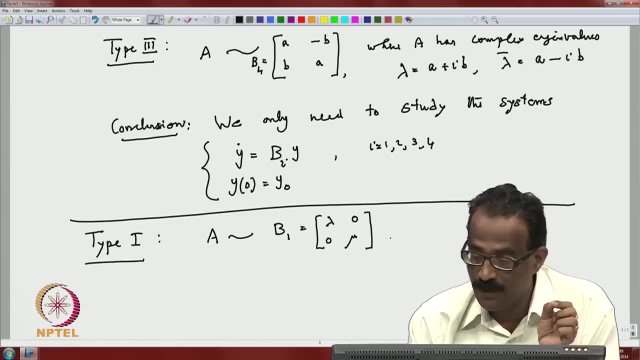 and minus beta 0, where it comes positive. Let me repeat it, you get into the other case. say the following example: A kid is failed and other kid fail and because of his Megabit, again recalling f, has two distinct taken values: lambda, mu, not equal to mu, and real. So we 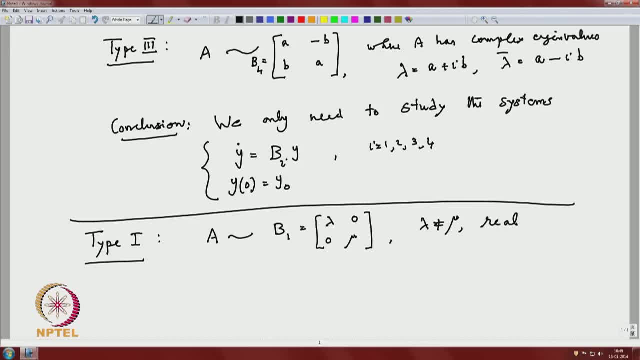 want to understand this thing. Now again we will split into various cases. So again we are putting the various case and we are assuming here also: determinant of whole analysis, right now. determinant of equal to 0. If the determinant of a not equal to 0, lambda and 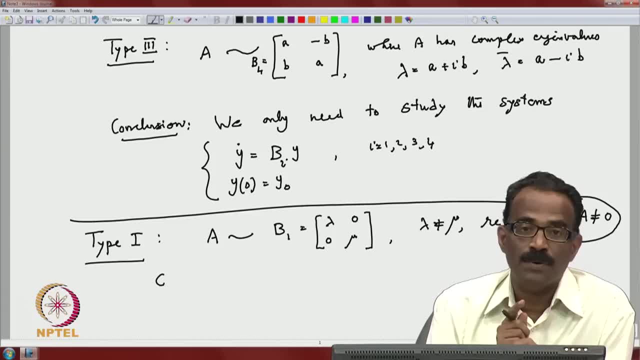 mu cannot be So. the only equilibrium point is the origin, no other, because of the invertibility of a. If one of them is 0 or two of them 0, then there will be many equilibrium points. So that are all special degenerate cases. We will give another two examples of degenerate 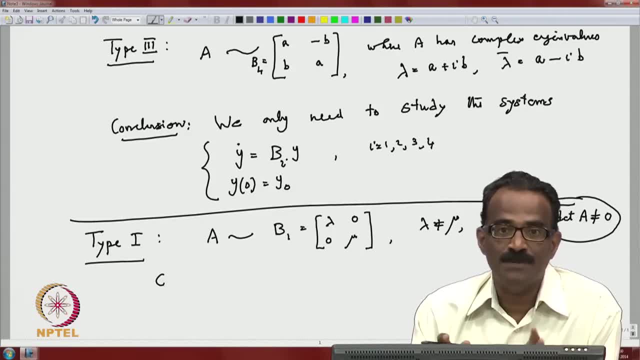 cases later. So we want to understand the situation where determinant of a So in the type 1, we have two classifications: Case 1,- this is within type 1, where lambda mu- the product, lambda mu- less than 0. So we will start with the examples and then you. 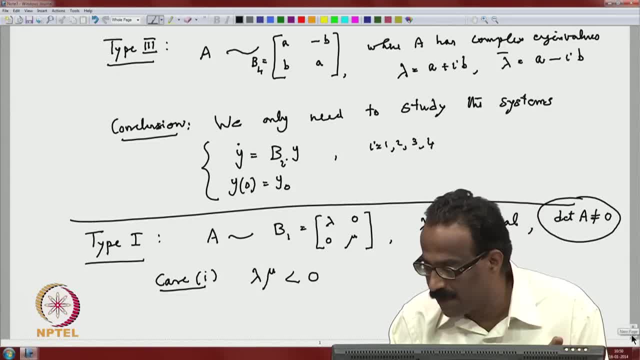 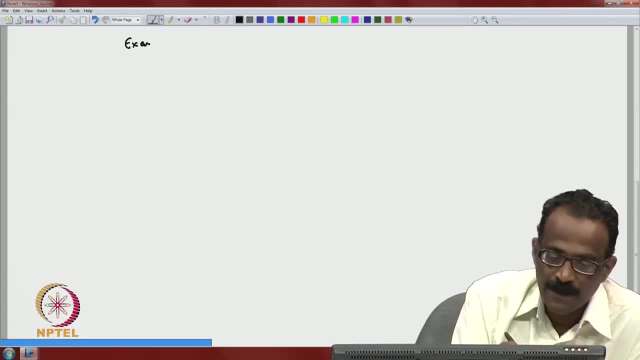 will see what happens thing. So let us take- we already seen one example, So similar example- we will try to see So example and then we will see that all All will work same way. So you want to understand the phase portrait, So we will take lambda. 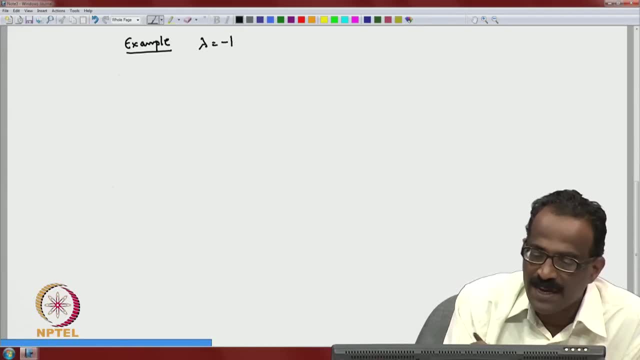 is equal to say minus 1.. We already consider such an example, but let me do it in a slightly sign. change How the arrows will change. Earlier we considered a saddle point situation. This is a saddle point situation with 1 and minus 2.. So it will behave same thing. So what? 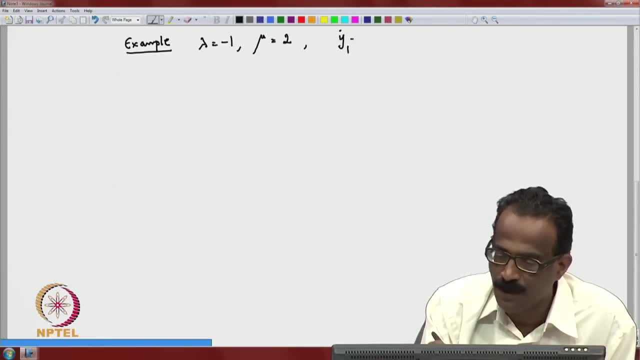 is the corresponding system, You will have y 1 dot is equal to y 1.. This we already studied, So there is nothing much to do. So we will take: lambda is equal to 1 and minus 2.. So 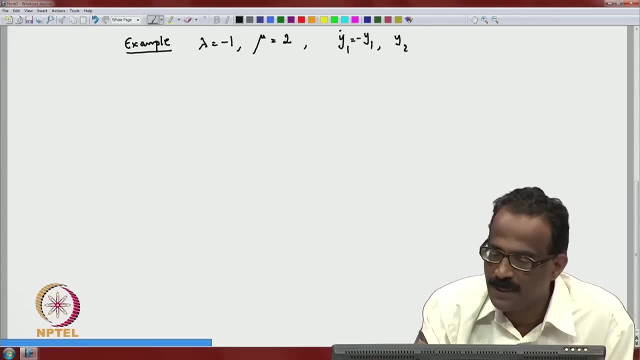 there is nothing much to do. it minus y 1.. y 2 dot is equal to 2 y 2.. You see, and you have your solution. I can immediately write my solution: y 1 t is equal to e power minus t y naught 1, and y 2 t equal to e power 2 t y naught 2.. This goes to 0 as t tends to. 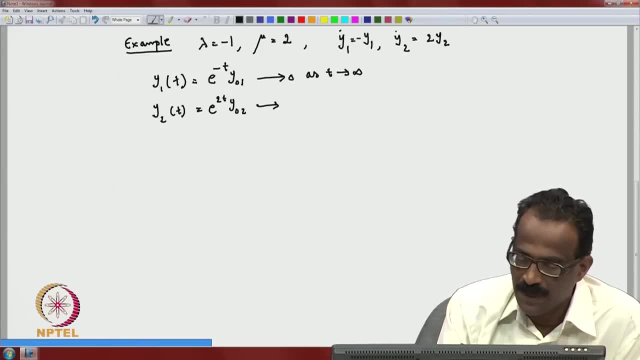 infinity. This will go to plus or minus infinity Depends of the sign of y naught 2.. y naught 2 is positive, Go to plus infinity. If y naught 2 is negative, go to minus infinity, as t tends to infinity. 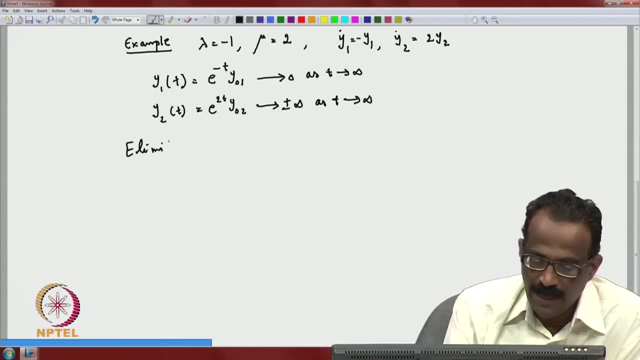 Eliminate x t. We have done exactly the same thing: Eliminate t, You will get it. You square it, You will get y. 1 square is equal to some constant with y naught by y, naught 1 by y. 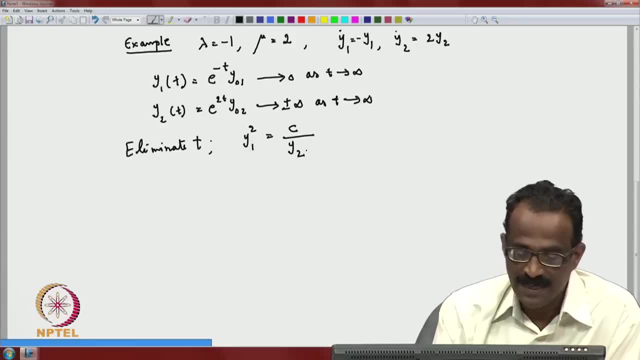 naught 2. Everything is constant. So now we take lambda dot plus all, So you can calculate constant into y, 2. So this is called the saddle point equilibrium, saddle point, which is an unstable equilibrium. Saddle point equilibrium is always an unstable saddle point equilibrium. 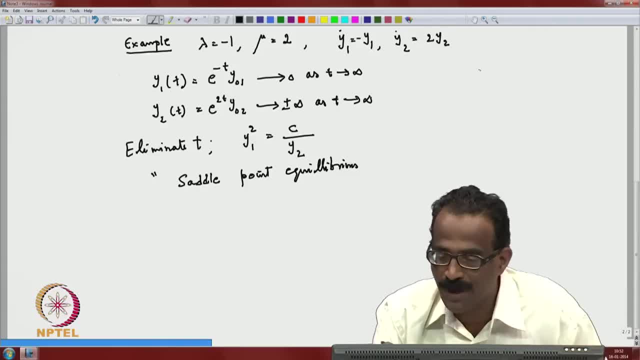 So if you plot your curve here, it is an exact thing. If you plot here, so this is a equilibrium point and y 1 is always going to 0.. So these things are here: y 1 part, this will be here, and y 2 going to infinity, so it will be here. it will be here, So if 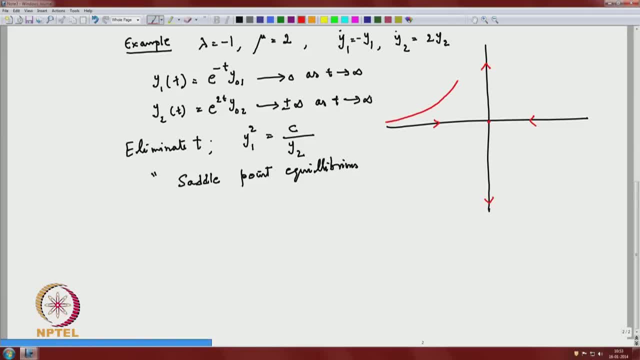 you plot your curves here now, so this will go to y. 2 is going to infinity, so it will be here. So this is your phase portrait plot here. this will be like this. this will be like this. So you have only certain cases. 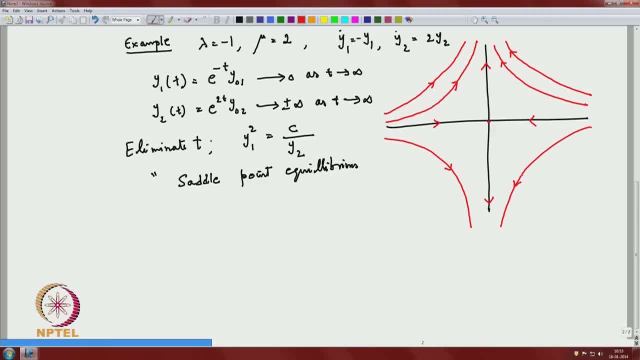 I will draw the entire thing after that. you should plot it accordingly. So, if you look at it, the x axis is called stable subspace, stable subspace and y axis. So you will define E as the stable subspace, E as set of all elements of the form x. 0 with x in r. 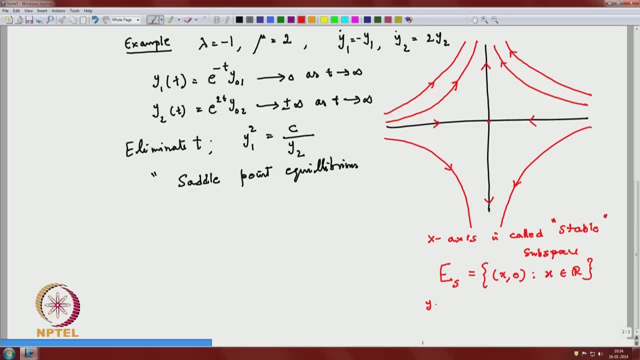 And y axis. unstable subspace is called unstable subspace. that is called E? u is equal to set. of all elements of this, 0, y, y is equal to r, And this will give you This, together, will give you your r. 2 can be decomposed into E? s plus. This is a general 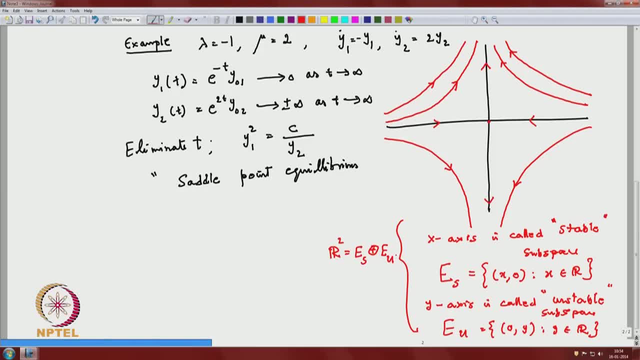 feature which we will see later: Every r and for a given dynamical system we can classify into stable, unstable. plus one more thing will come note when you go to this thing For the shaded point. this is the case: you can classify thing. You can also. now you 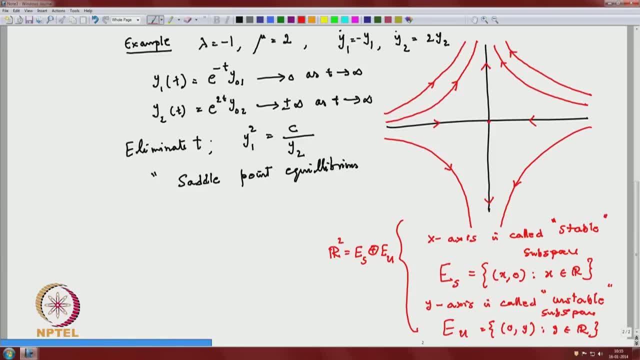 also know how to plot your, How to plot the vector field here. So this is the phase portrait. in this situation, by taking lambda equal to minus 1 and mu equal to 2.. What I am going to say, tell you, is: 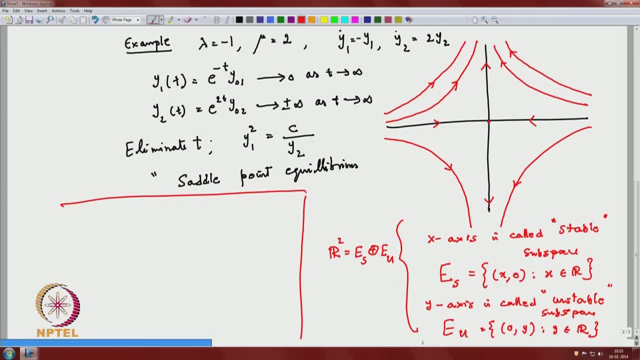 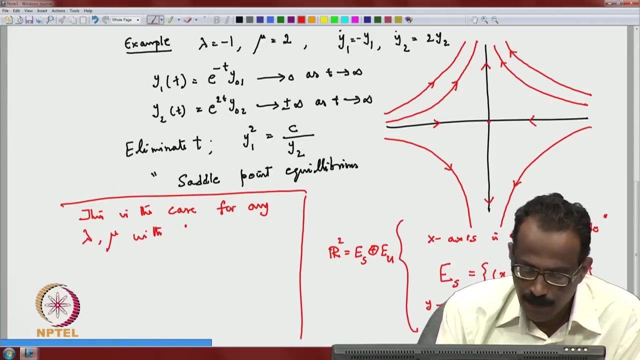 that this from here. it is not anything specific about lambda and mu. What you need is a different sign. So this is the case. this is the case for any lambda mu, with lambda mu negative. that is what I am saying, If lambda and mu have. 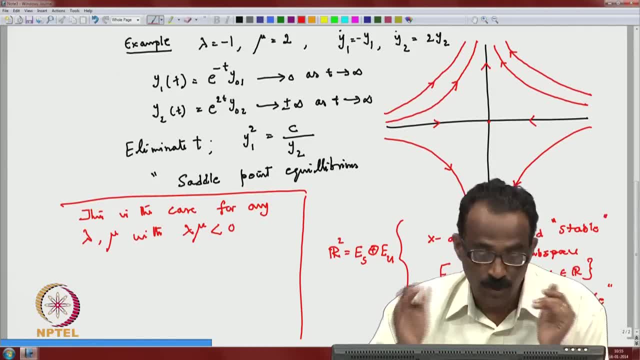 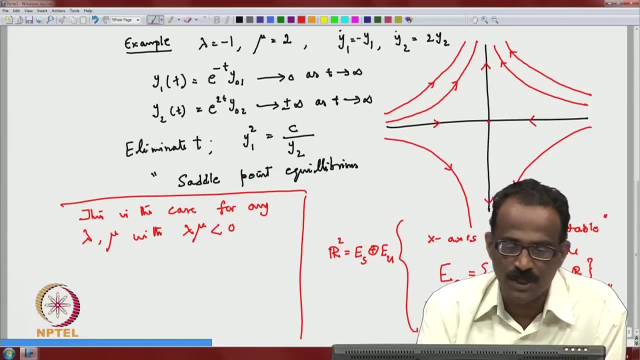 opposite sign. this is case one within type 1.. So whenever you have two Eigen-value is real Eigen-values distinct, but it will have different sign. you can do this one instead of y 1 t power míos t by naught. you will get e power lambda t y naught 1 and y 2 t. 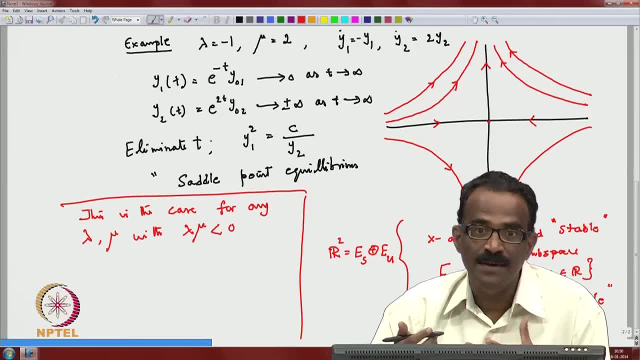 will be e power, mu 1 by 0. You can write The mutual caracterization. that is why this ganzen property is from Let something saying to go multimedia what I can write. So I mu t y naught 2.. Then, if you eliminate t, you will have an expression of the form some. 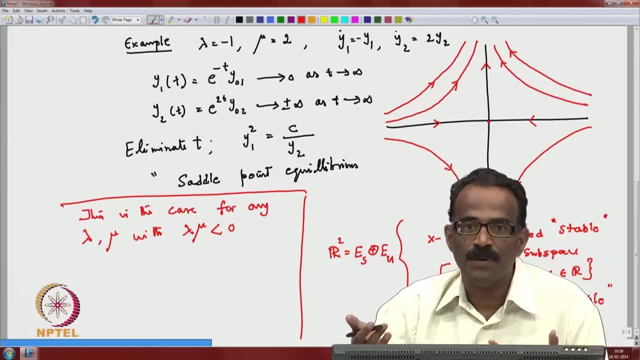 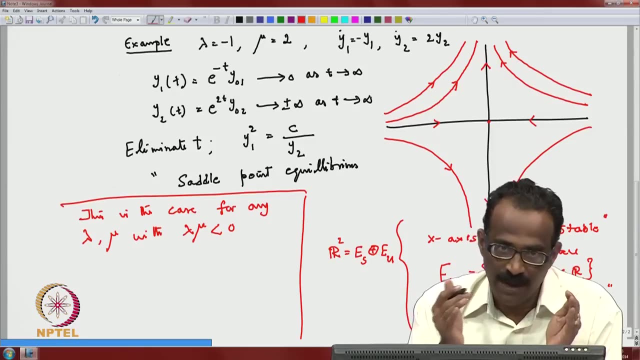 y 1 power. alpha is equal to c by y 2 power. So the trajectories will be the same. It will remain the same way. Only thing: depending on the sign- which one is negative, which one is positive- the arrows will change. You will have one directional arrows with lambda. 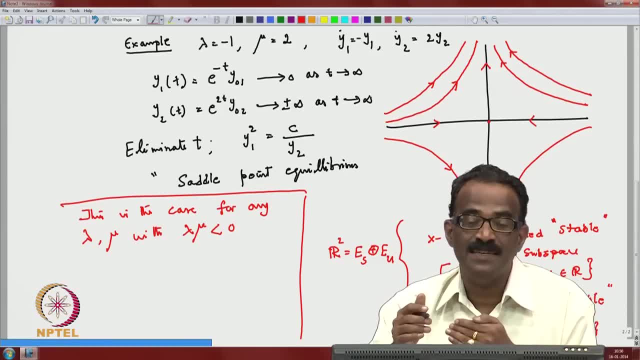 negative and mu positive, The arrows will change. if lambda negative and mu positive, The stable axis- either x axis will be the stable in this case. In that case y axis will be unstable, or you will have x axis unstable and y axis stable. So this gave the case. 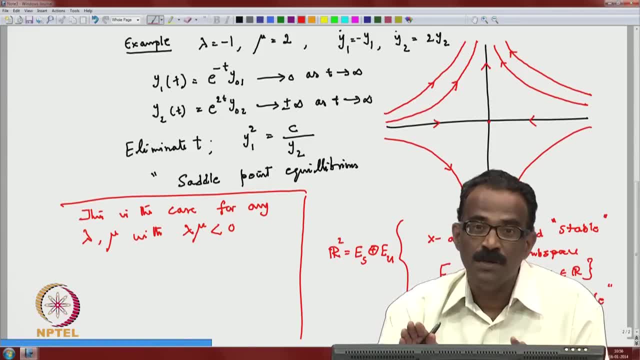 for all type 1, with distinct Eigen values, with different opposite sign, will have this sign And all these equilibrium points. in this situation of lambda mu negative is called the saddle point equilibrium, So the behavior will be the same as saddle point equilibrium. 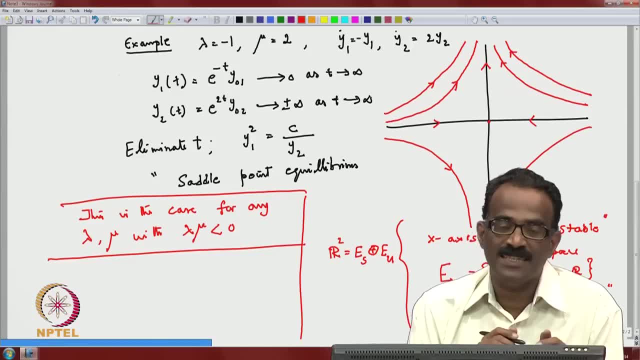 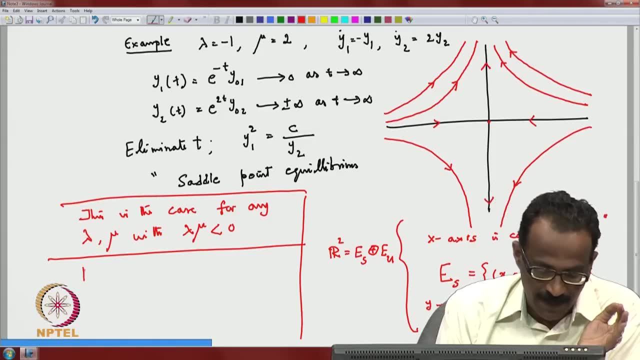 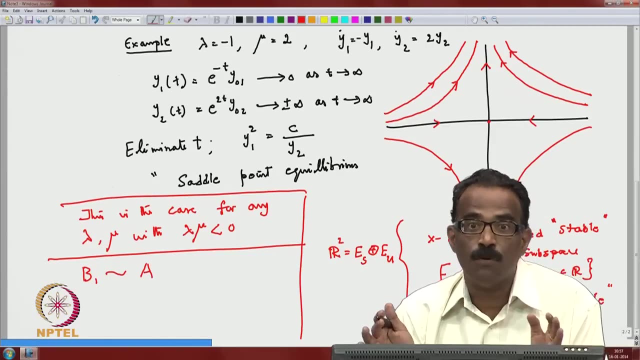 One more point I want to remark here before going to the next case. If you make this linear equivalence, if you have this particular matrix B 1, which came from a linear equivalence A 1.. Similarly, this is just a change of coordinate system. So instead of having this thing corresponding, 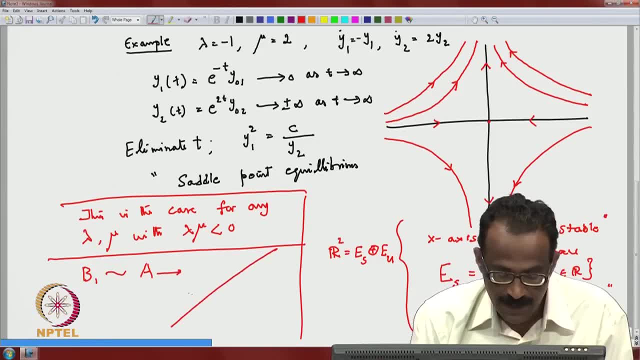 to A, you will have a new coordinate system, something like that. You may have a another coordinate system, Need not even be perpendicular, but again this corresponding point origin will still remain, because under linear equivalent there is only one equilibrium points, which 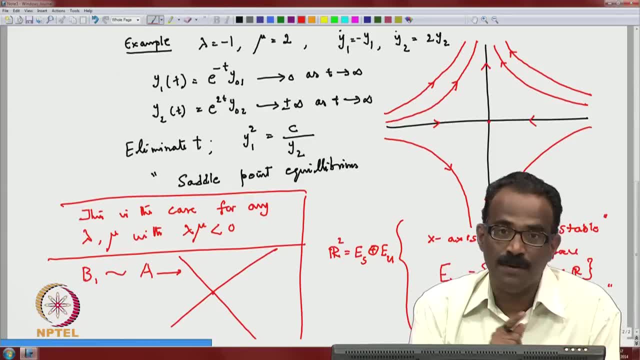 is the origin, And the origin will still remain because of the equilibrium points. In that case there will be a coordinate change and your trajectories will still be like that. You see, the nature of the trajectories will be like saddle point, equilibrium with. 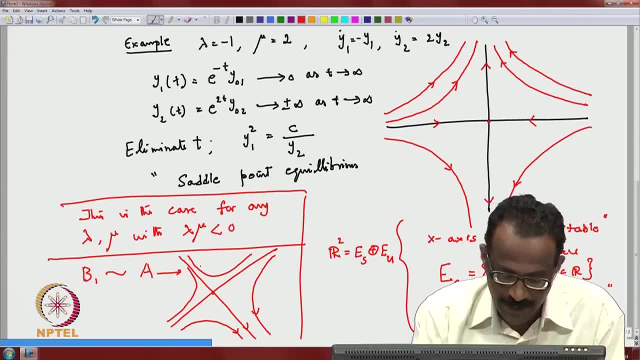 appropriate the arrows, You have to put appropriate arrows. That is all That will give you, depending on the sign and thing. So all here and this will be in this direction, you see. So that is what I said. There is no difference in the nature of the trajectory. 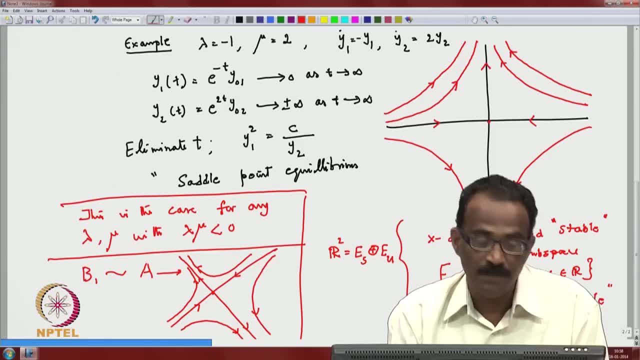 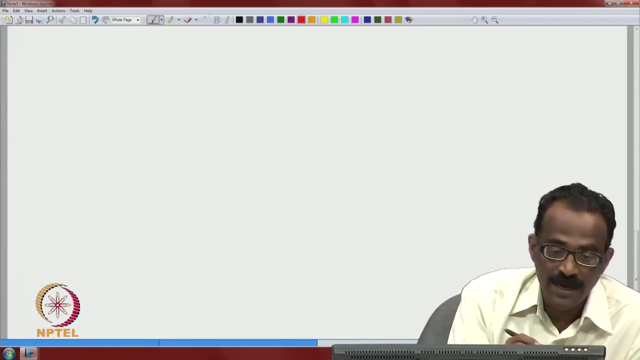 Nature of the saddle point, nature of the equilibrium point. for all the matrices, all coming from B 1 or B 1, corresponding to the matrix A with lambda mu less than 0 will have the same nature of the solution. So now go to the type 1.. And type 1 again, with lambda. 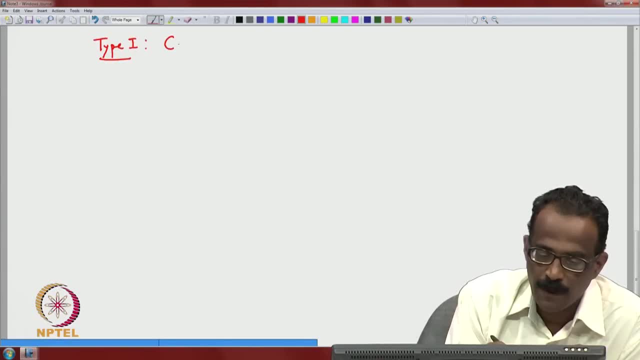 mu. So this is the case 2 with lambda mu positive. You see, that is the case. What we had seen is that with lambda mu negative. Now, within this there are two cases. You see, there are two cases with lambda positive, mu positive, And there is another case with lambda negative. 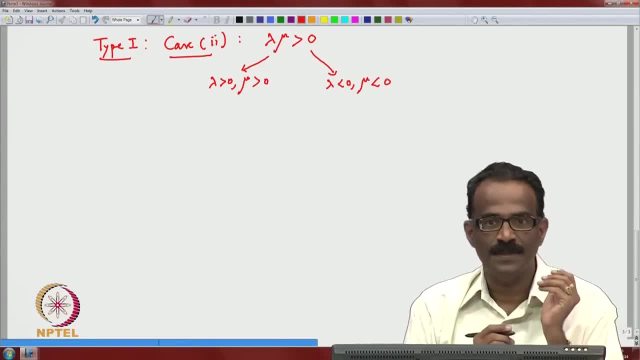 mu negative. You have to understand both these cases. So the best way again is to take up the example. It will behave in the same way. So let us take start with an example. So this is the case again, B 1. So you start with example. Then you will see that there is no difference. 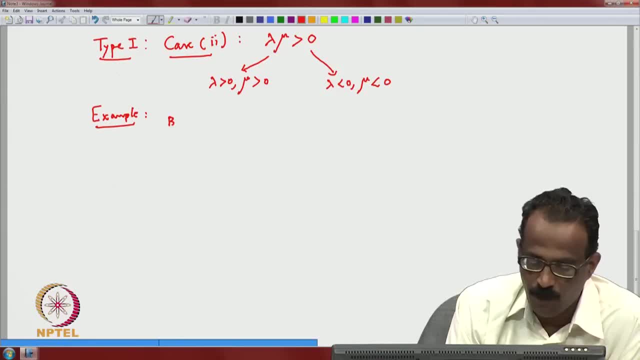 example, You take B 1 to be of the form. It is all in the case of B 1 type 1.. So you take to be 1 0, 0, 2. You take it, You want the form. So you take B 1 to be of the form. 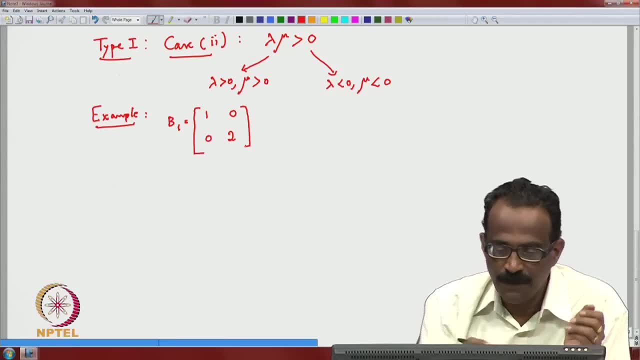 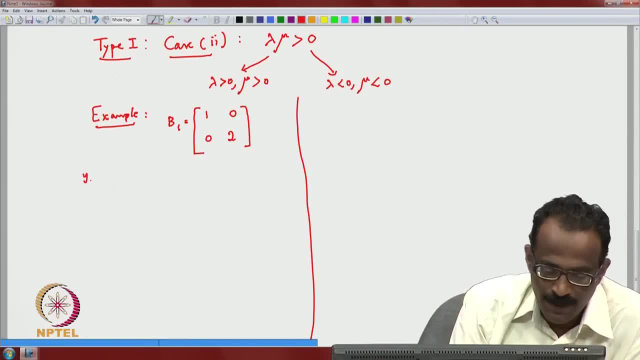 If B 1 will have, you can write down your solution. Your y 1 t will be e power t y naught 1, and y 2 t will be e power 2 t into y naught 2.. See, in either case, this will. 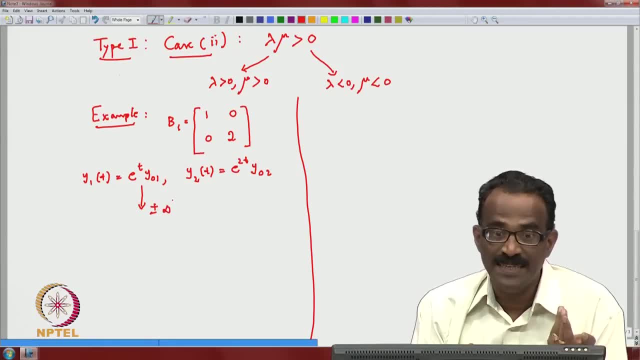 go to plus or minus infinity. e power, t minus, depending on the sign, this will also go to plus infinity. Now, if you eliminate here, your y 1 square will be constant into y 2.. This is something like a parabola. 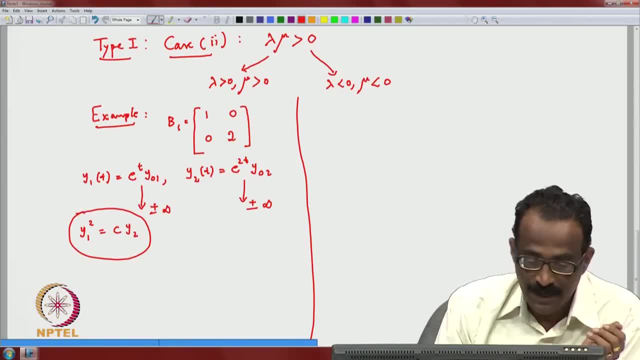 You see, so you have a parabola thing. So if you plot this curve here again, look at it here. Let us look at our first equilibrium point. This is an equilibrium point. This is a decoupled system, So if you start from here, it will remain in the same axis. It. 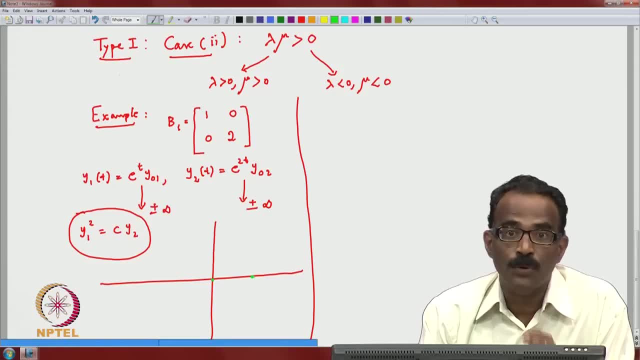 cannot move because if it is in x axis, your y naught 2 will be 0 and y 2 t will be 0. Hence it will remain in the x axis, But then y 1 t goes to infinity, because y 1 t is equal. 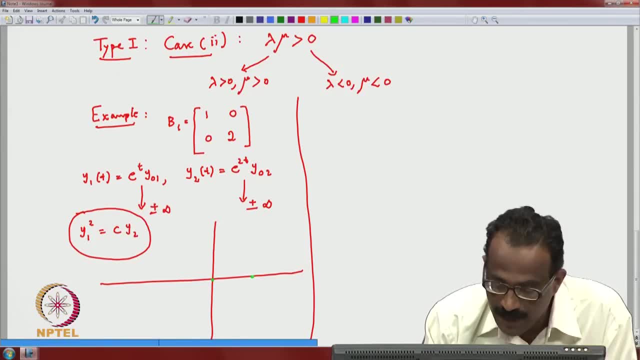 to e power, t into y, naught 1.. So the arrows will go. It will move along this direction. If you move from here, it will move away from here. If you start from here, it is the same situation, but both Eigen values are positive. It will. 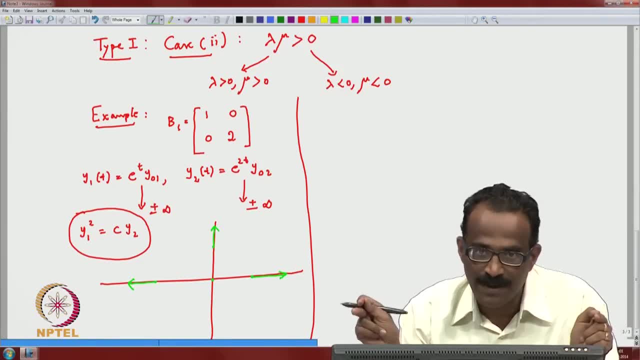 move in this direction. In the saddle point equilibrium, if one axis moves away, the other axis moves towards it, but in this case both moves here. So if you move here, it will be something like that. So it will be like that. What about if you start a point here? 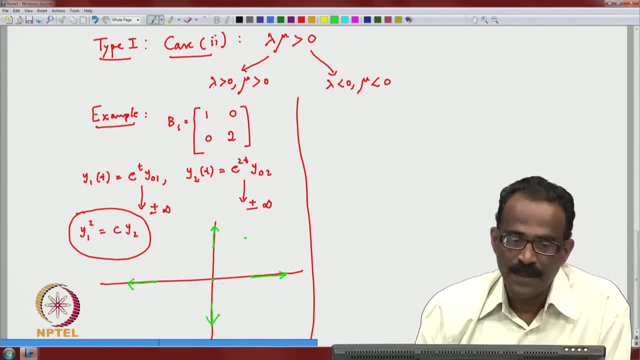 If you start a point there, both y 1 and y 2 goes to infinity, but it moves according to this rule. That is something like a curve, which is something like a parabola. So as t tends to infinity, it will move along this direction. This portion will be the t because 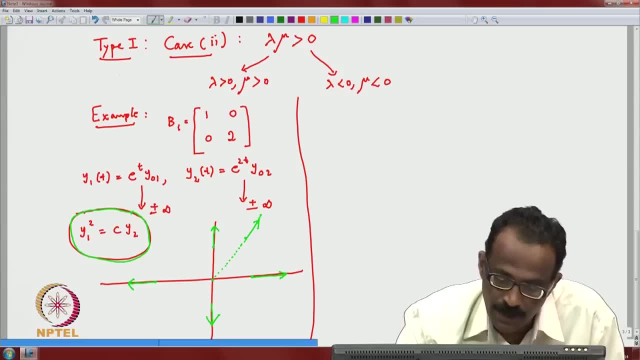 the solutions are defined even for the minus infinity. So it moves along these curves. So if you start from here, it will again move. So it will move along this direction. It will again move here. This is for the t positive side and this is for the t negative. 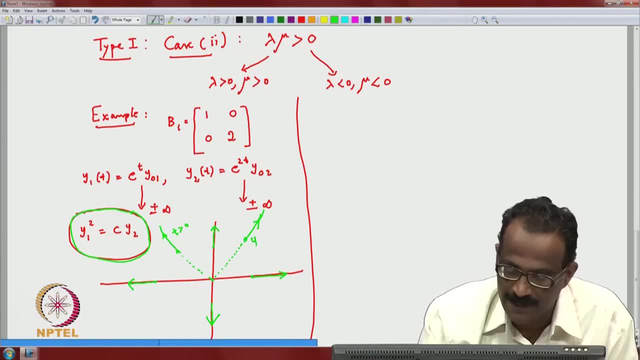 side. At this point is your y naught at t equal to 0. Why not At t equal to 0. This is for the part t negative. So from here, if you move again, it will move along the parabola. This is the region. So if you start from here, it will move The. 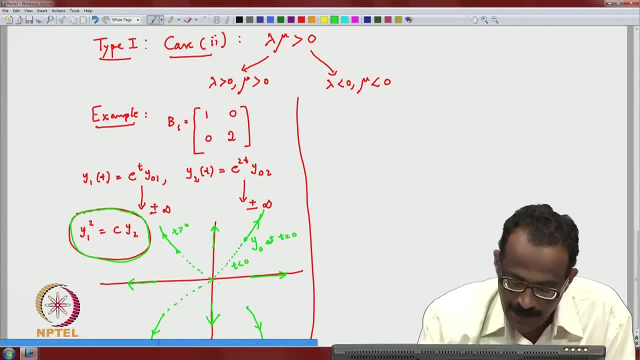 parabola may change it. What I am trying to say is that this is the same situation for any lambda mu positive. Same case for any lambda positive. Only thing is that e power t You will have. e power lambda t y naught 1.. Y 2 t will be e power mu t y naught. 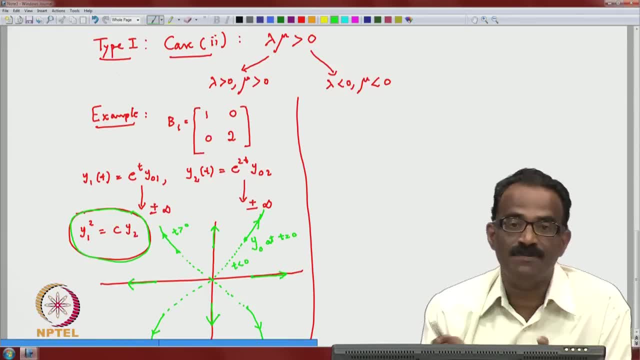 1.. So you may not get a relation: y 1 square is equal to c y 2, but you get a relation, something like y 1 power alpha is equal to c y 2. So y 1 square is equal to c y 2, but 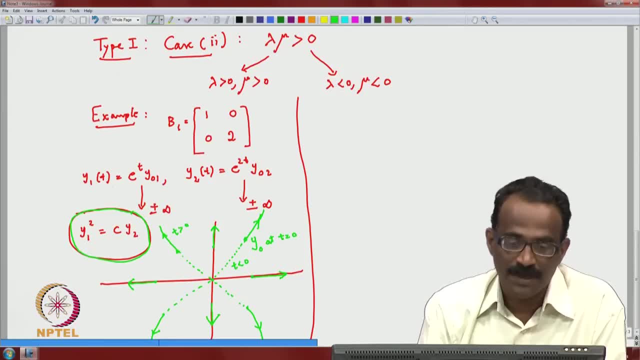 y 2 square is equal to c y 2, but you get a relation, something like y 1 power alpha. So is equal to c y 2 bar beta thing. but the curves may change, the behavior will be same. Such a point is called the equilibrium point is called a node equilibrium, equilibrium. 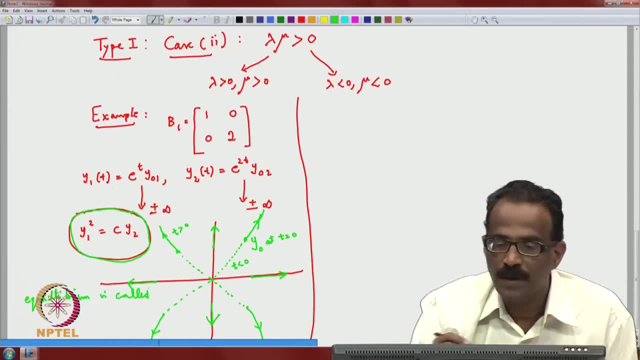 is called. let me write down this one: node n, node e- and this is unstable- is called. a is an unstable node because, whatever be the solution, any point you start a solution here, solution will move. however close it is does not matter, it will move. So of course, the 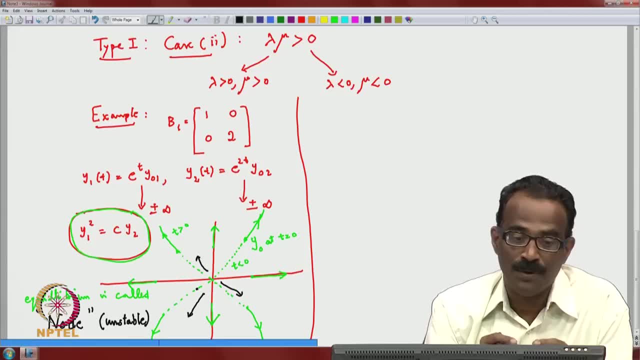 trajectory will change. So, whatever be the close point y naught closer to the origin, the solution will. trajectory will be- and this equilibrium is referred to as the node and what I am saying- that this is the same situation with any lambda mu, for all lambda positive mu, positive this curve. 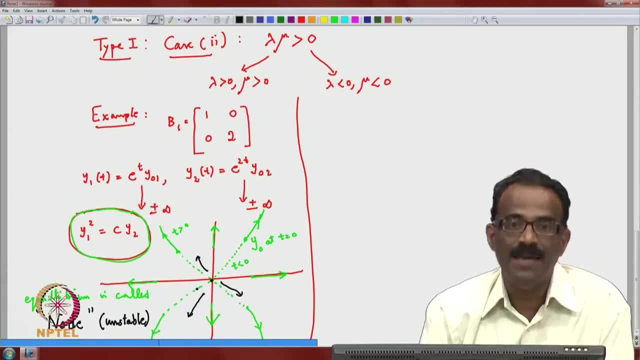 will be, the behavior will be the same thing. Now let us look at this case. So in this case, if you look at it, you start with the b 1 and then say: look at this with b 2.. So both with minus 1, 0 and 0 minus 2, 0 say both. 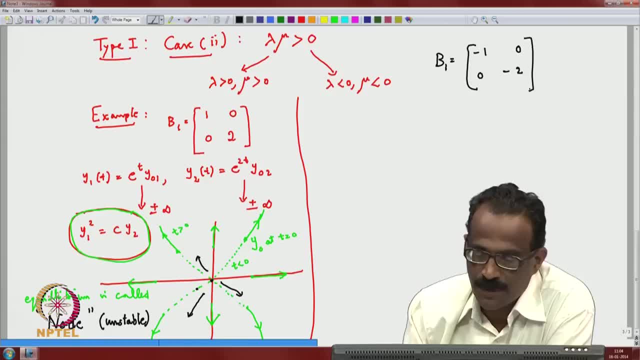 with minus 1, 0, zero minus 2. you want a system, So the corresponding systems you can write, So you will have your y. 1 t is equal to e power minus t y naught. 1 i to t is equal to. 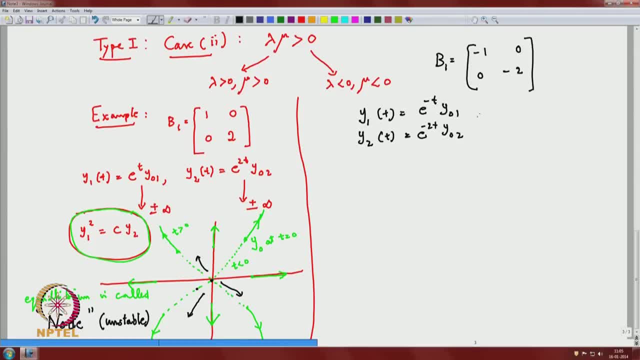 e power minus 2, t, y0, 1.. So if you eliminate you will get a gain. y 1 square is equal to some constant into y 2.. The only thing you should know is: if I have a linear system, then three eigen implications: 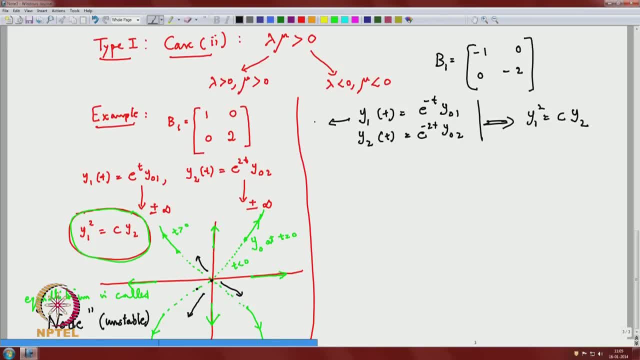 P. mimic some quantities to this diagram to stands for a number of cases. if I have g as, the only thing is that this will go to 0, both will go to 0 in this case. So if you plot this curve, the curve will be the same. So you have your equilibrium point. So in 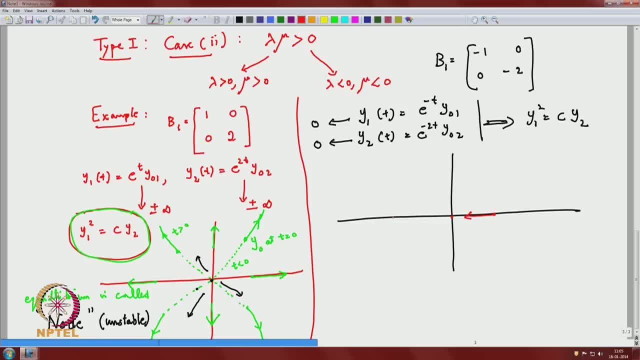 this case, if you start from here, only the arrows will change because it is going to be 0.. If you start here, you will have here So the curve from. if you start here now, this will come towards the origin along that. you see, This is the negative part. So this: 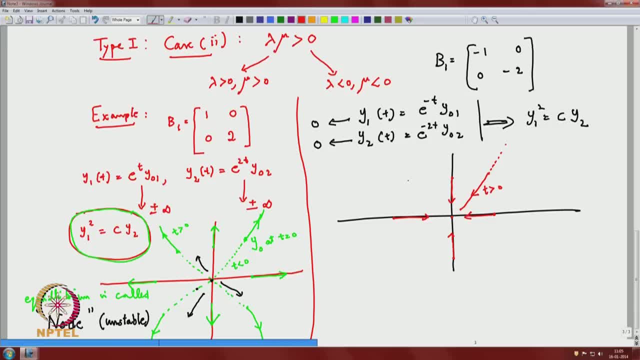 is the positive part now. So if you start from here, so it will here. This is the t positive part. So this is so. if you start anything from here, any point does not matter. If you start from here, it will go to the. it will only go as t tends to infinity. So 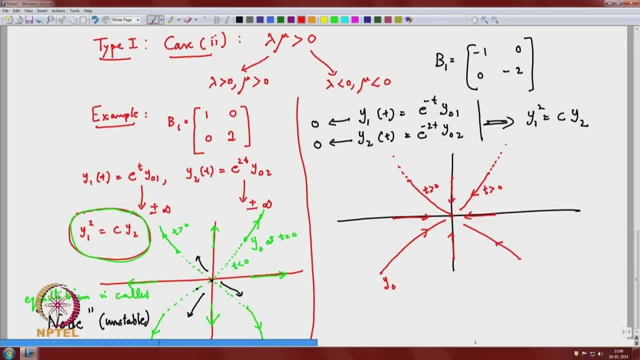 if it is the same thing, it will go to infinity. So this is your phase portrait as an- and this is again a situation of a node. In this case we call a stable node. You will have this stable node and you have a. 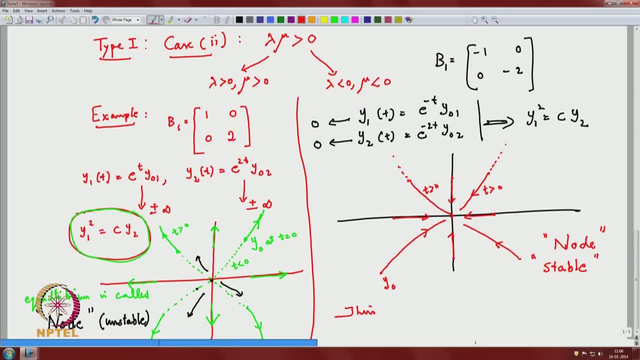 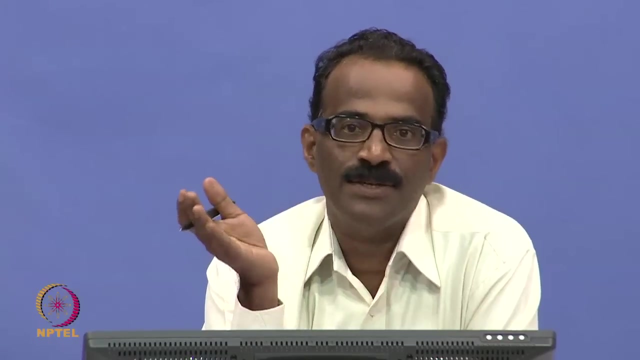 So you start from here- is same for all, lambda mu with lambda mu. So what we have done is that in the type 1, when it has two distinct Eigen values- lambda mu, negative- you have a saddle point, equilibrium, which is unstable. One trajectory go to 0,, one trajectory go to infinity, or 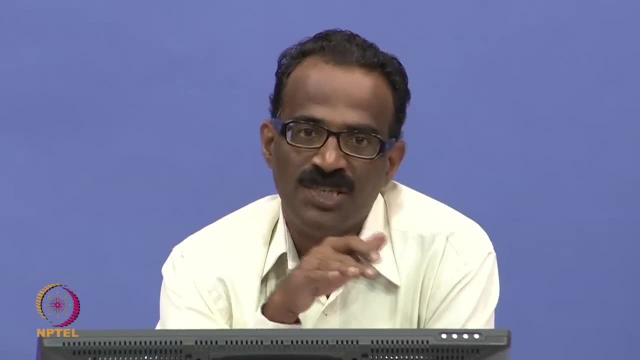 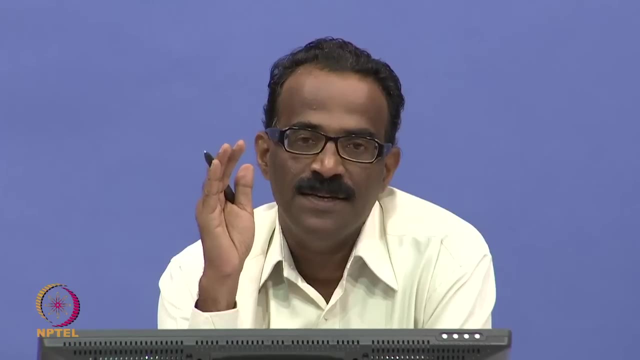 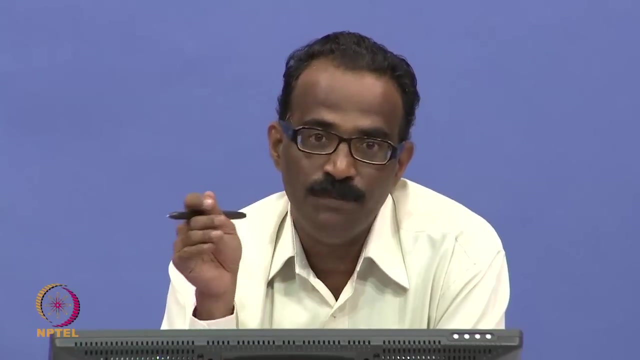 minus infinity. When it is lambda mu positive, either both trajectories will move away from the equilibrium point, going to infinity, giving an unstable equilibrium. On the other hand, when lambda mu positive, with both lambda and mu are negative, both Eigen values are negative. 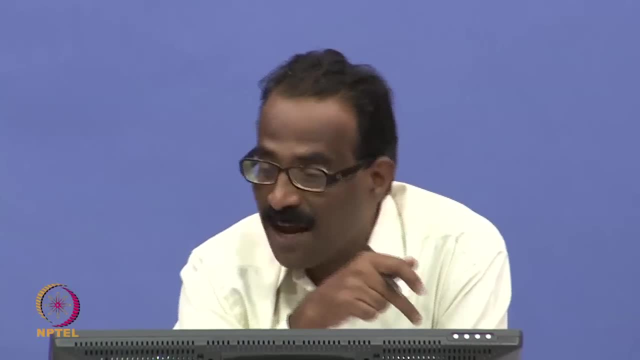 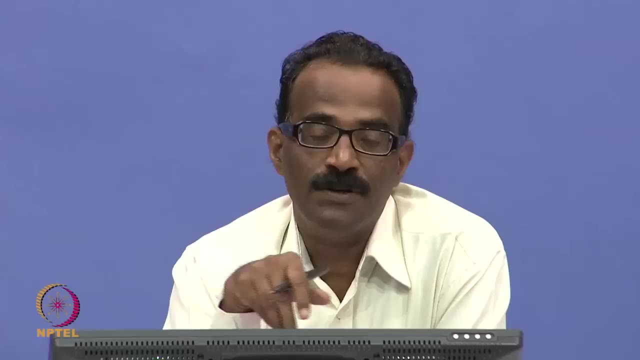 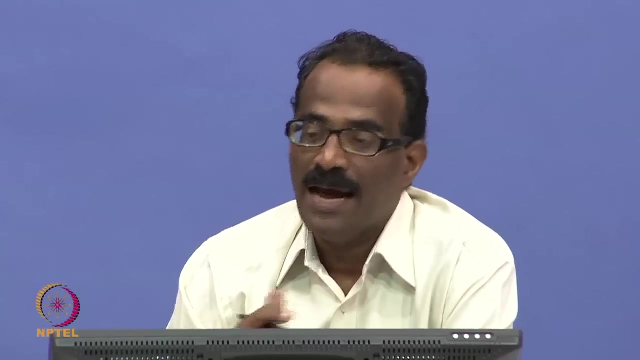 then the solution trajectory will go to. in fact, it goes to the origin in an asymptotic way, giving a stable equilibrium, And we refer to this case with lambda mu. positive is a equilibrium point is called a node, And your subspace, in the unstable case, the whole. 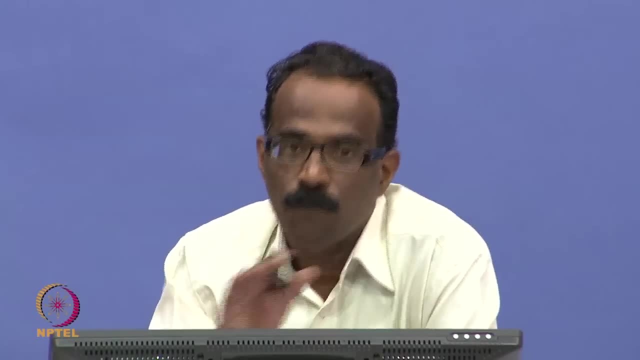 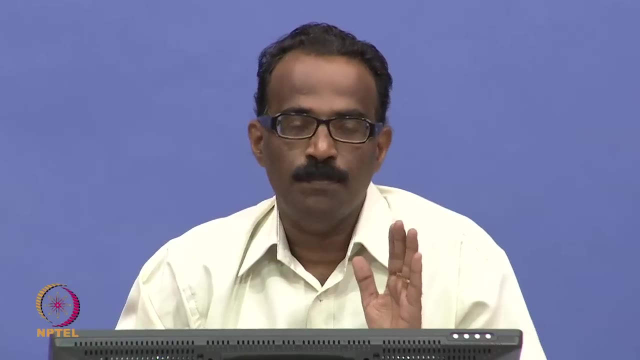 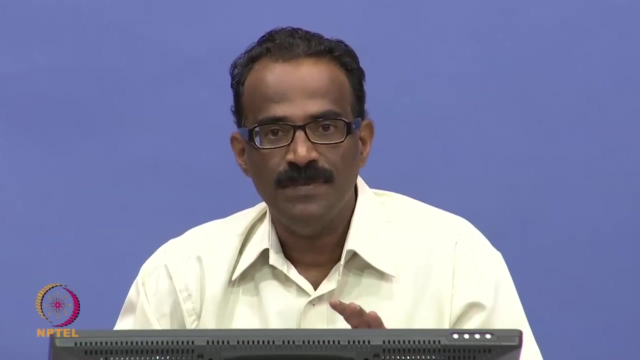 R 2 is an unstable space In the stable thing whole. R 2 is a stable case. Now in the next class we will continue with this for the other two cases of type 2 and type 3.. What you are going to see is that type 2 more or less behaves like in this fashion.